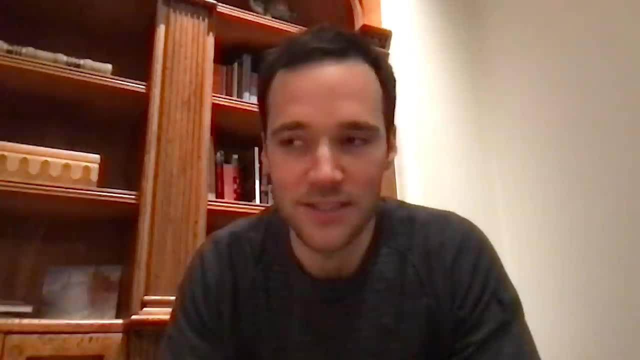 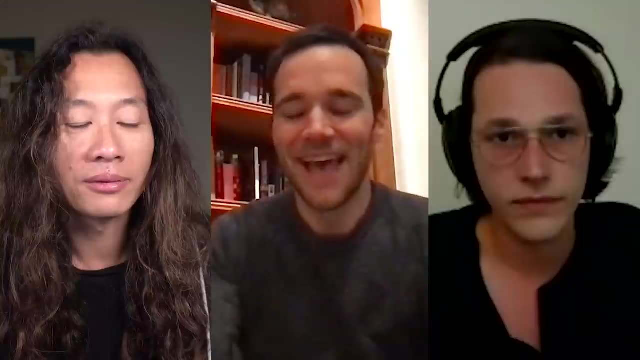 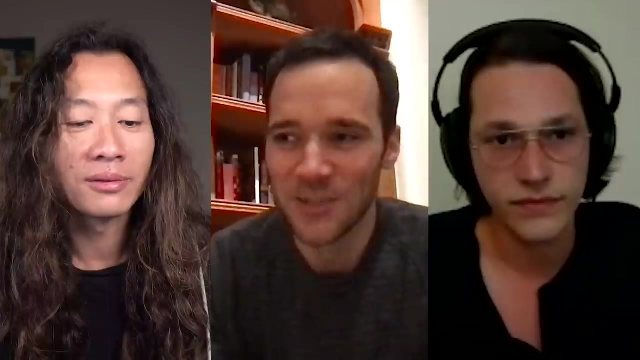 talking about crypto and we were both really interested in the solana ecosystem and um and ended up co-founding fractal together. uh, super excited and uh, well, we'll talk about the- the story of of the fractal launch, but also the fractal nft launch, because that was sort of a 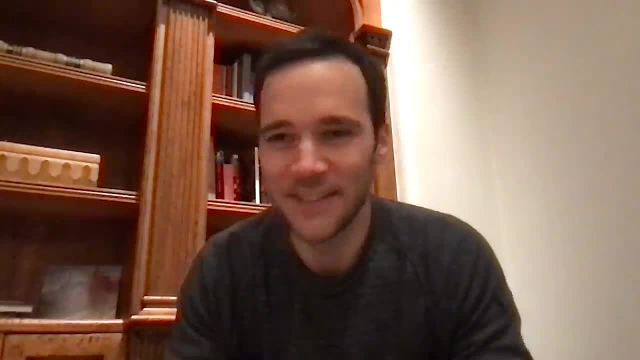 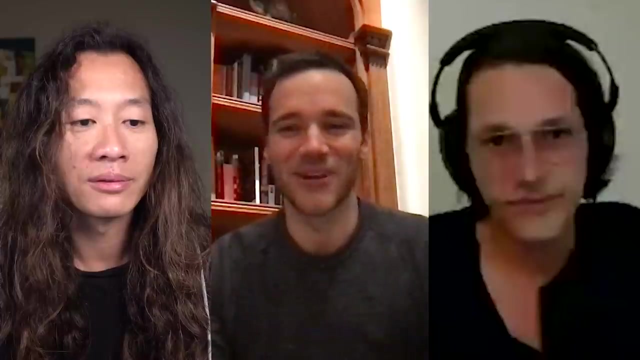 surprising organic um idea we had sort of spontaneously with with the community and it was quite a ride to try to prepare the largest solana nft drop by a factor of 5x in just 10 days. so we're excited to share the story and um to be joined by ludovic, who um who helped us pull it off. 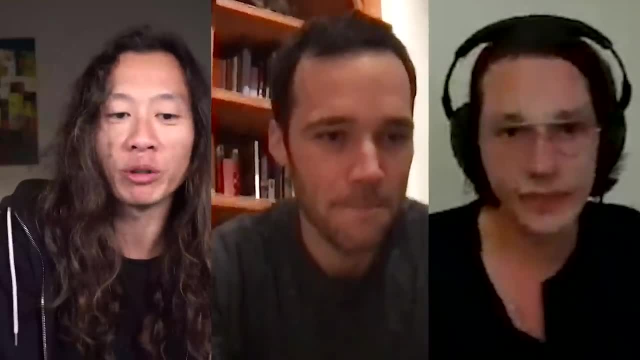 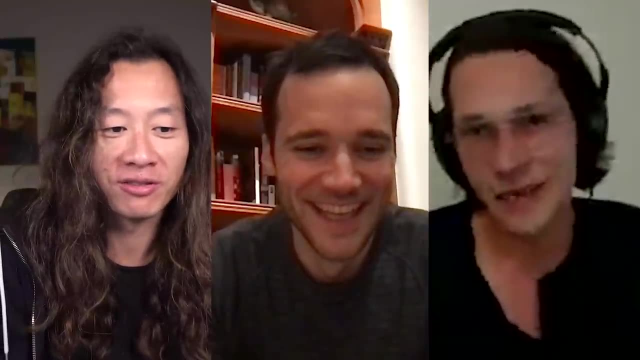 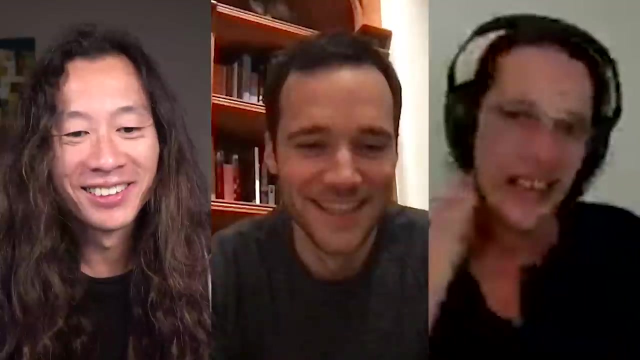 yeah, ludovic, you were recruited. you'd work with dave before right, and then he recruited you to to do this and he tells me that you are an actual particle physicist. yeah, well to be. uh, to be fair, it's a physicist, so like theoretical physics. but yeah, my background is in physics. i know i work as 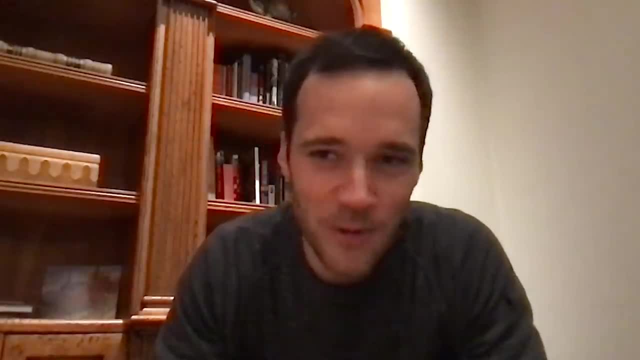 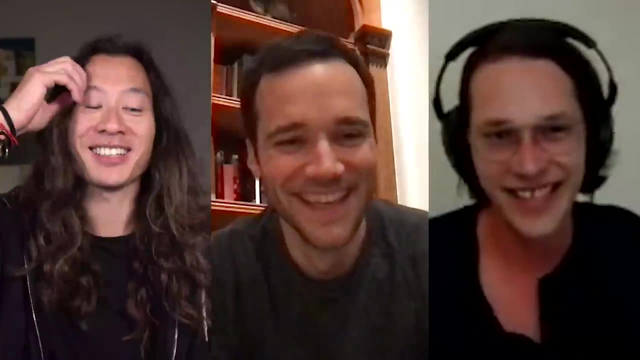 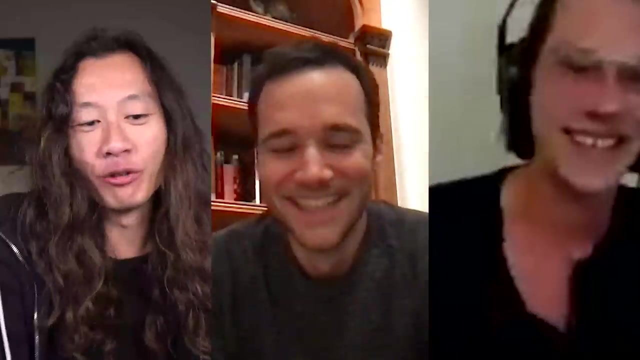 a data scientist? yeah, ludovic. ludovic is the smartest guy i know, justin. he's very um, you know, he's very humble. that's, that's saying something. you're surrounded by eggheads at google, weren't you? i'm just kidding, um, so tell ludovic, tell me, you have some interesting. 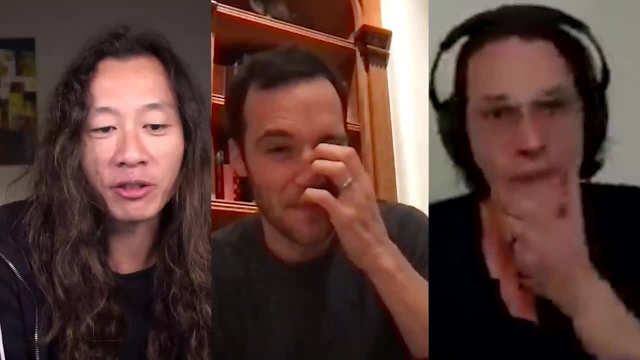 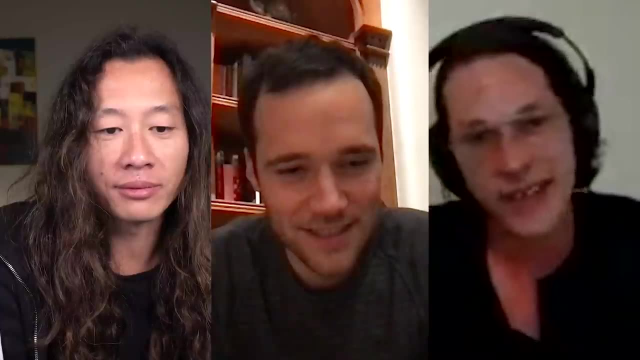 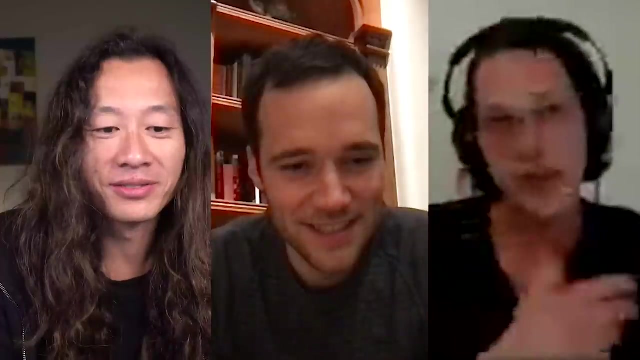 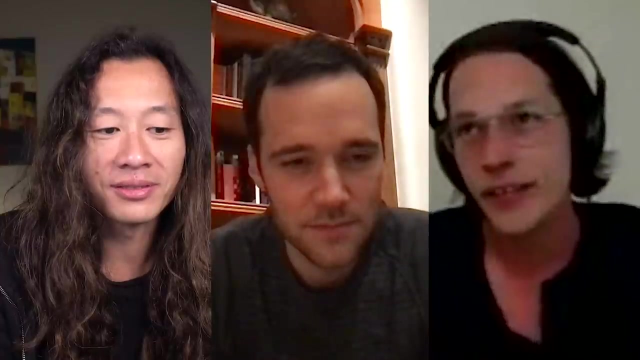 crypto back stories- crypto background. tell me, like, uh, how you got into crypto. yeah, i got. i got in uh into crypto. that uh dogecoin crave, uh, where uh people started creating all sorts of altcoins- they were not mineable by asics, but mostly like so, uh, by late like 2013. uh, one of one of my friend, 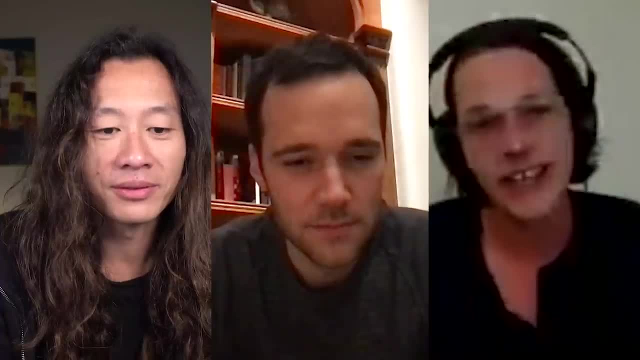 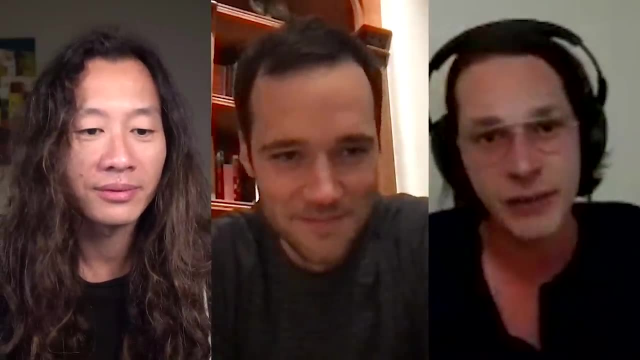 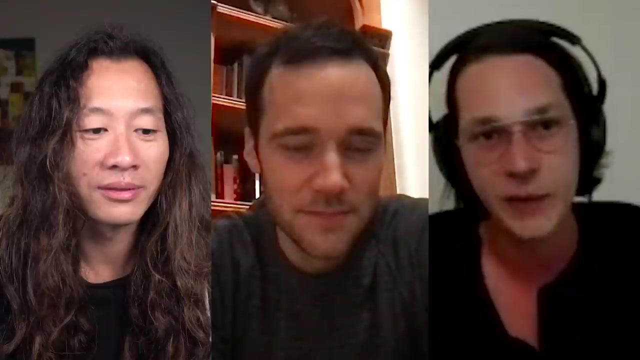 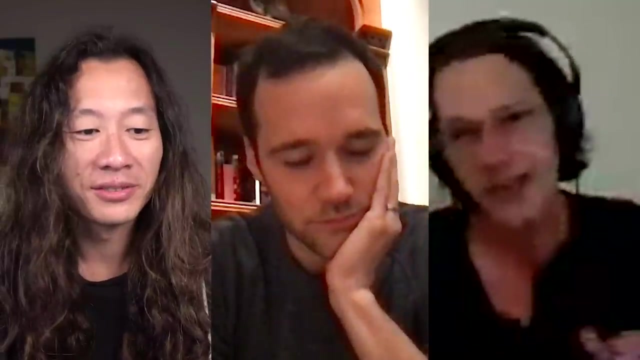 and i, we uh, we built a rig and started mining and so on and, uh, we got really excited even during day trading, and that's all. also, i lost all my crypto because the exchange, uh, where i was doing, pretty much closed down and they ran off. that. wow, oh no, that was like, uh, early entrance in crypto and an early exit as well. 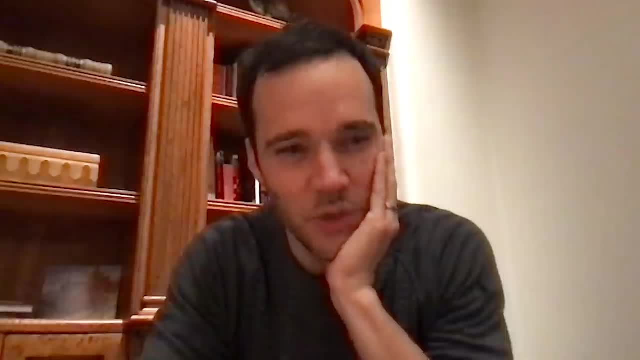 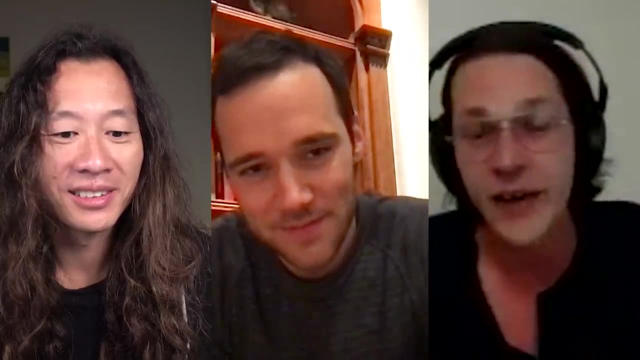 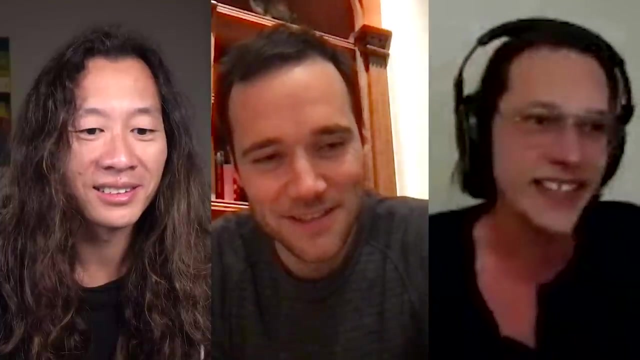 then i i focused more on my uh you like wrote, you wrote crypto off for like years. right, yeah, i didn't want. uh, i heard about f, uh ethereum very early. i was like, yeah, smart contracts, pretty interesting stuff, but i still didn't want to invest because i was kind of a- i had a bit of a kool-aid hangover. 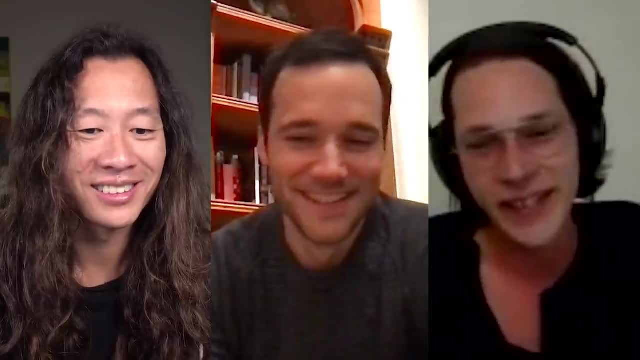 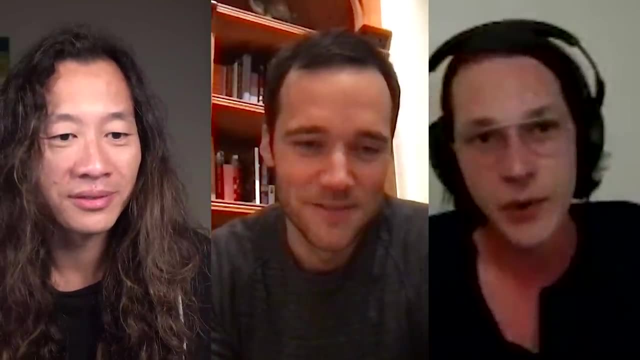 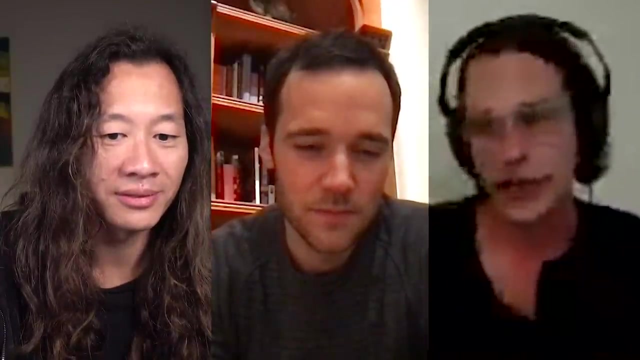 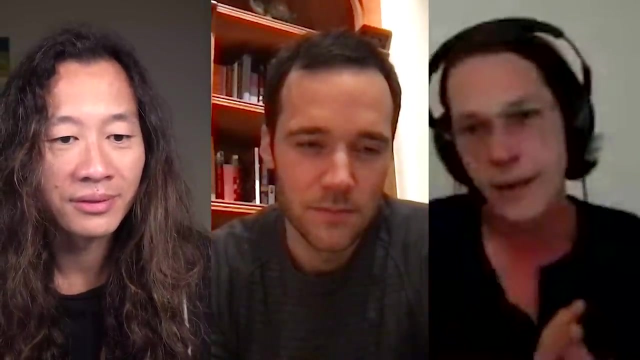 let's say yeah. so uh, that was kind of a yeah, my story with uh with crypto, but, like more recently, with the more like a recent project with the crypto economy, the tokens, and not creating a hundred but actually creating ob coins on on the same chain as another crypto. um, that's very interesting and instance is very interesting in terms of just the. 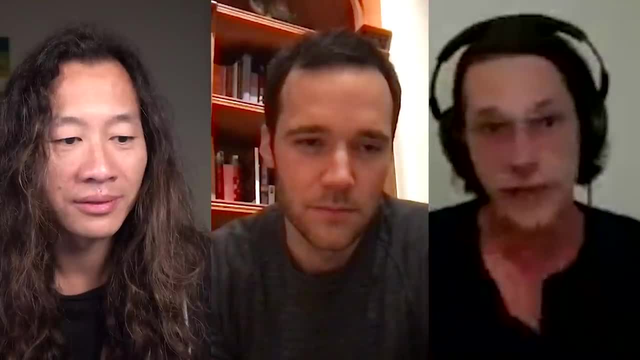 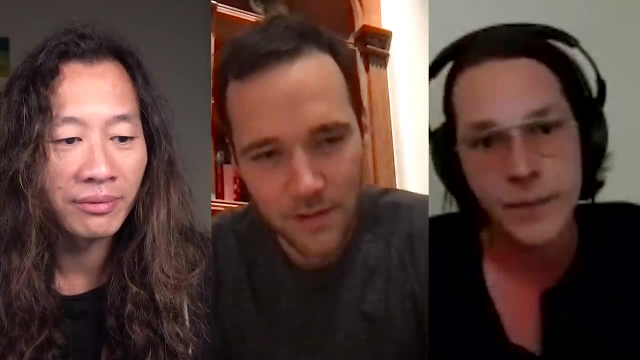 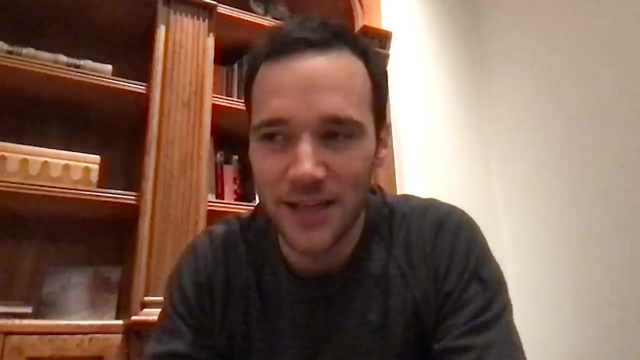 the algorithm and the algorithm mix that's behind it. That was one thing that convinced me that, yeah, crypto is cool again and we should do something with that. So Ludovic had told me- just an interesting fact about Solana- that as you approach the speed of light, 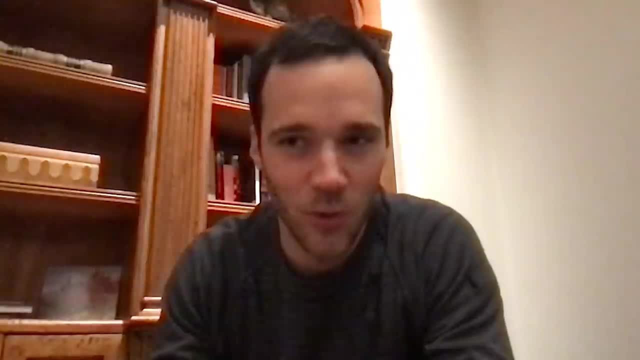 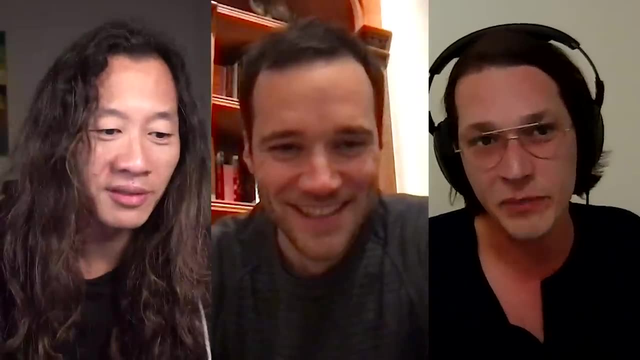 the physical phenomena behind proof of history, which is this core underlying tech of the Solana blockchain stops working. Is this right, Ludovic? Right, right, right, Like I didn't prove that, but I suspect that because of relativity. 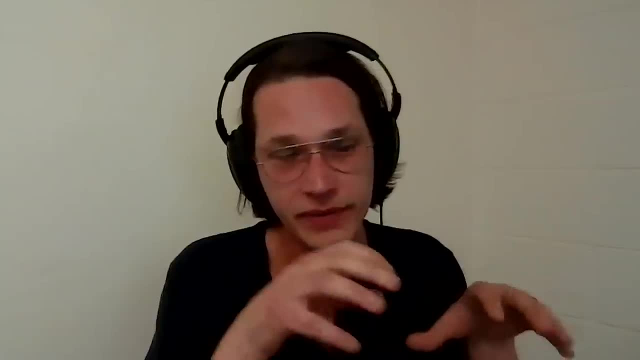 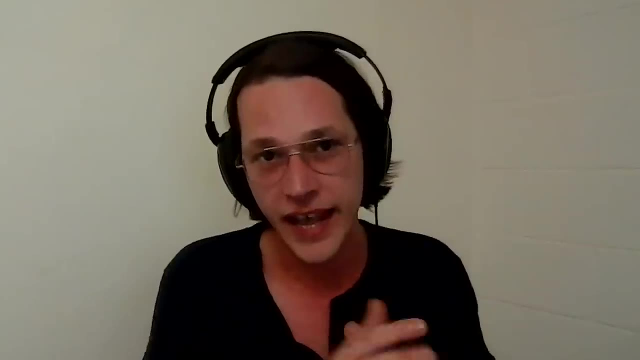 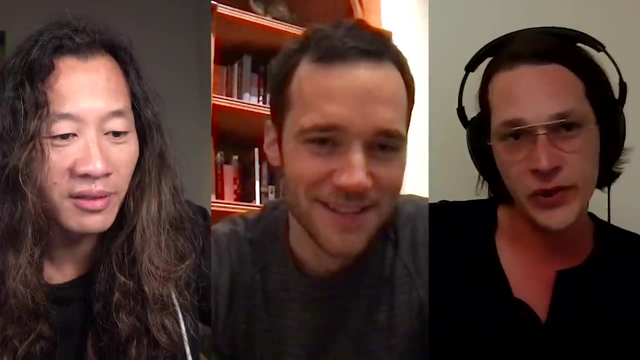 things that are not casually like in terms of causality, that are not related together. they might happen in any order, And I'm not sure that the proof of history on Solana is causal. And so if you were to put a computer in the sky, 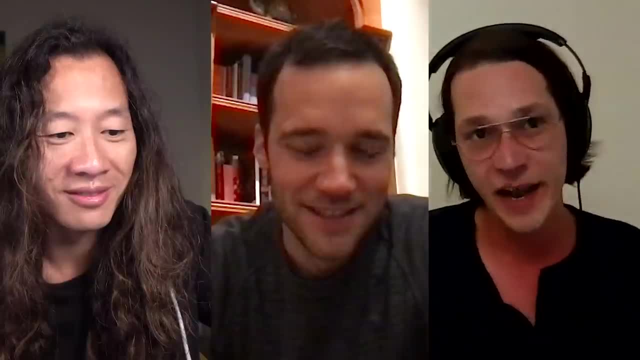 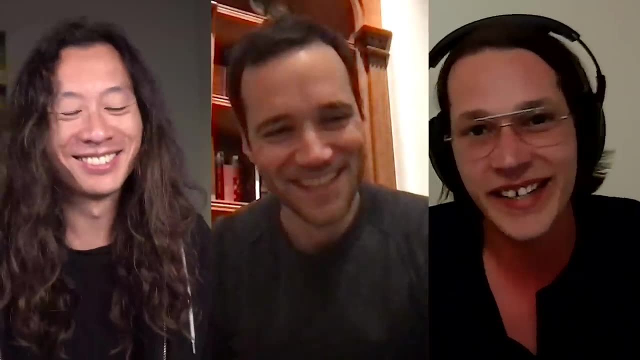 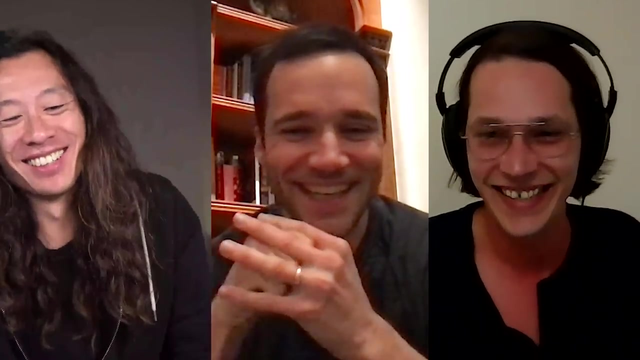 on a satellite and had it travel extremely fast. I think you could actually try to attack the network. So maybe in a thousand year we should consider that for Solana We're gonna have to upgrade. Yeah, Okay, All right. well, let's dive into Fractal. 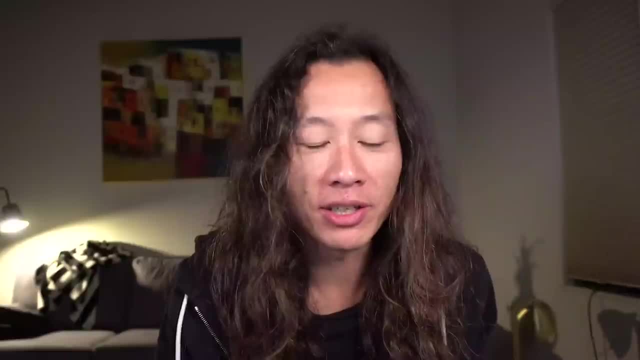 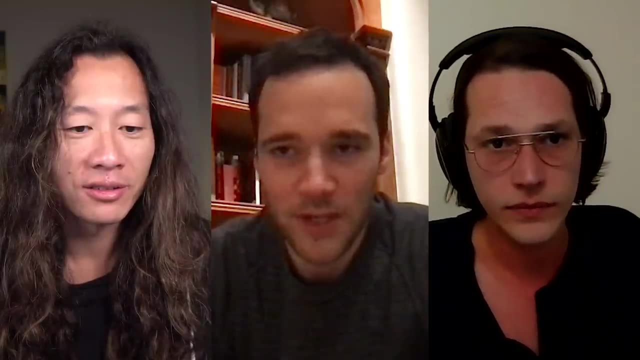 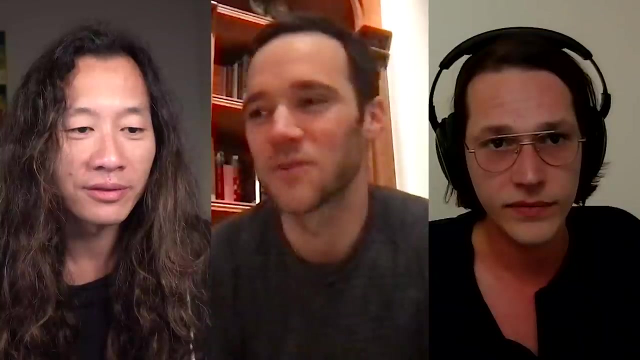 So tell us about the collection, David, and like, how did we come up with it? Yeah, so our Discord was growing pretty quickly And our community was asking for anything- a token and some type of drop, And so, of course, we're gonna make our community happy. 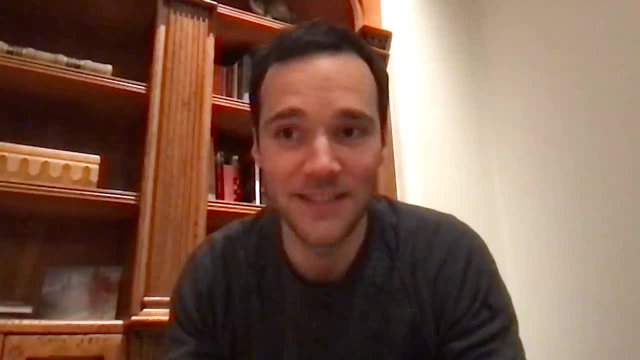 So we decided pretty quickly that we were gonna drop something to them, an NFT specifically, And at first we thought this would just be a token of our appreciation for joining the community early. you know no big deal. Pretty quickly after we realized we had a big opportunity. 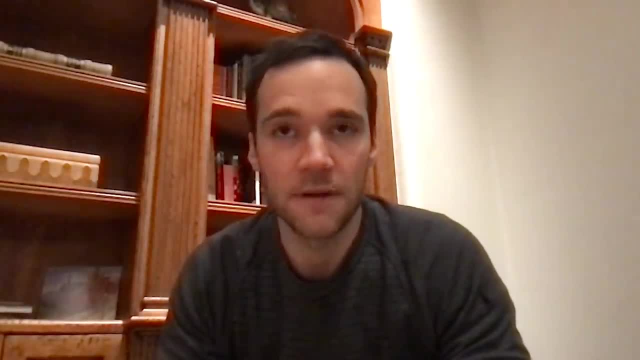 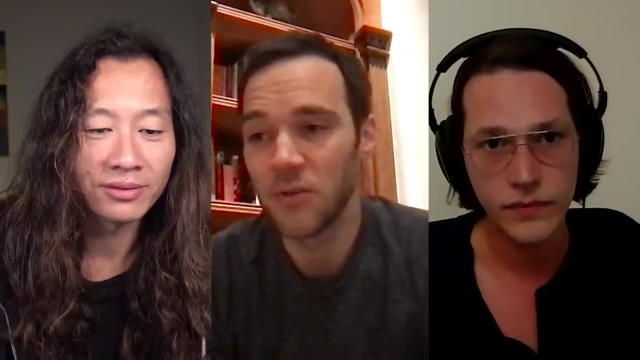 The Fractal community was, you know it was, you know, being built from folks that were new to crypto. you know, from Justin's network, from Twitch. Many of these folks in our community are new to crypto, new to NFTs. 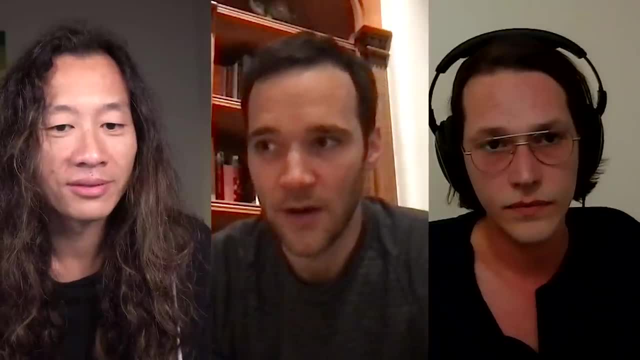 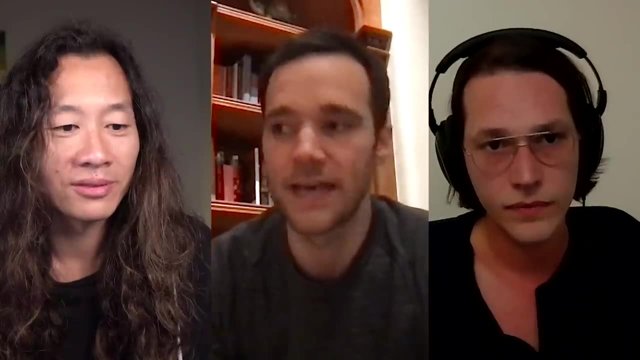 And one of the futures that we're excited about at Fractal is this vision of a Web3 gaming world where you own your own assets, And one of the things that falls out from that is that you can use the same assets across different games. 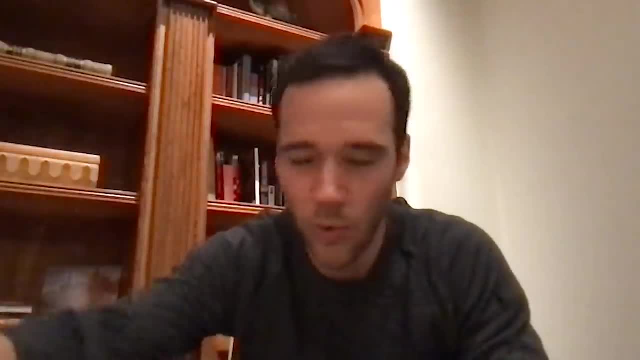 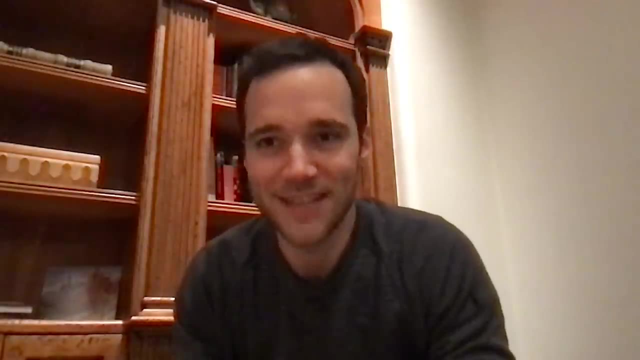 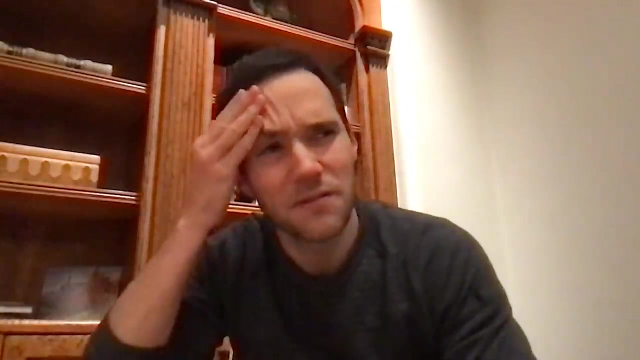 So if Ludovic owns a special sword in game one, he could potentially take that out of game one, bring it to game two and wield it there, And that is a really exciting potential way in which Web3 games could work. And so we sort of like: 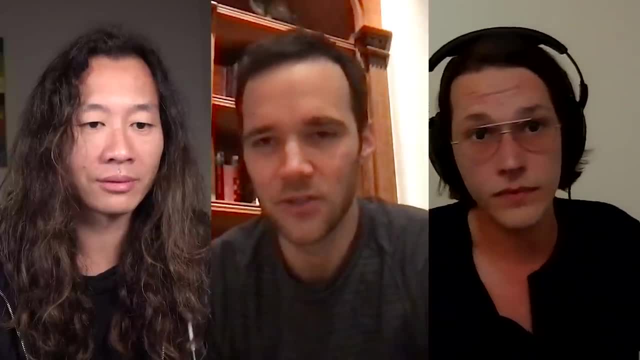 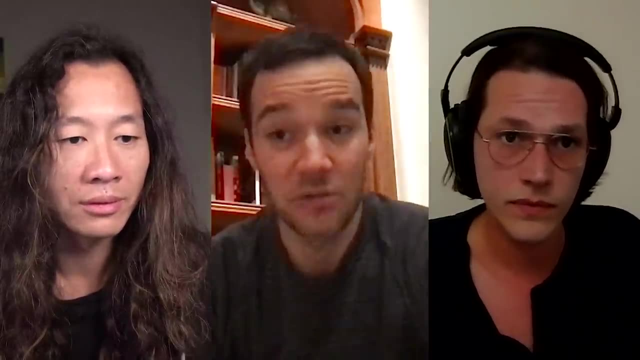 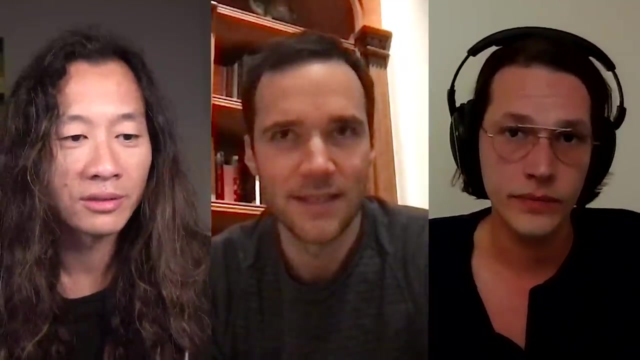 realized that with this really awesome, engaged, diverse, inclusive community that we were building in our Discord, that we could actually drop an NFT that could show this potential Right, we thought to ourselves: why don't we build this primitive, if you will, for power level right? 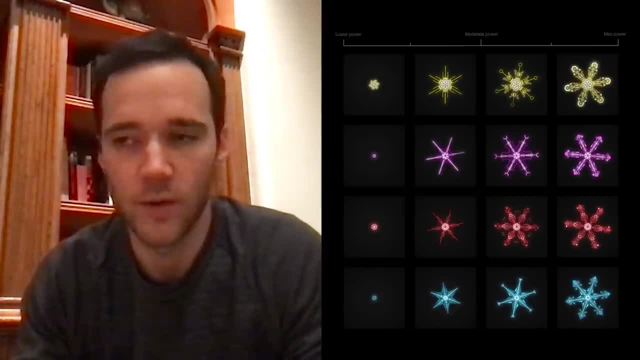 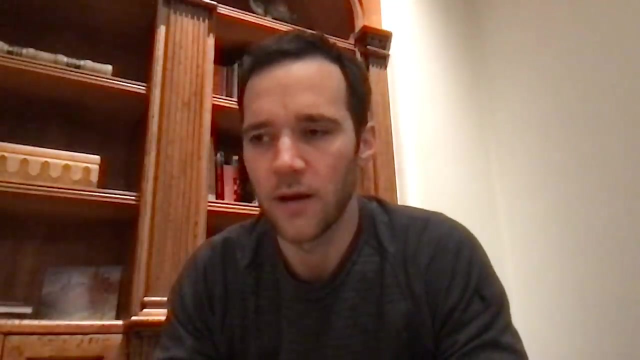 Power is something that lots of games have. There's always a notion of you know how much energy you have, right? And we thought to ourselves it'd be really neat if we had this cross-game power primitive And similar to you know, like the loot project on Ethereum, where 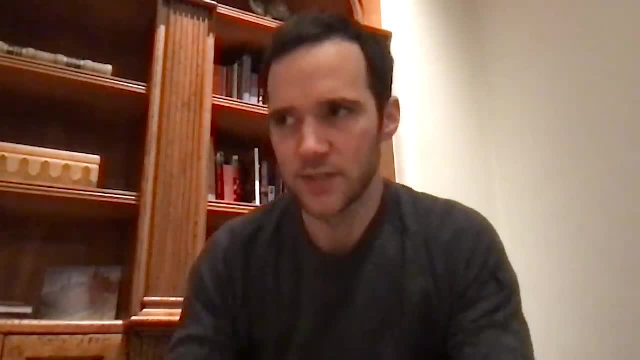 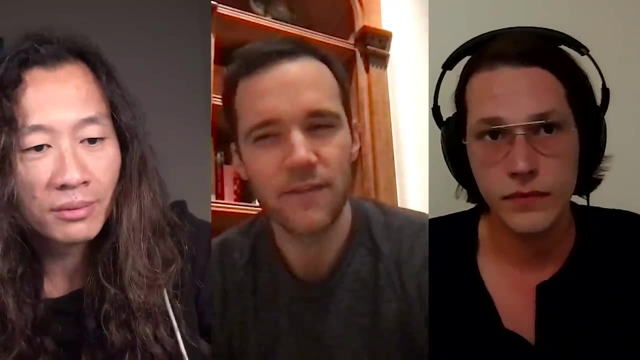 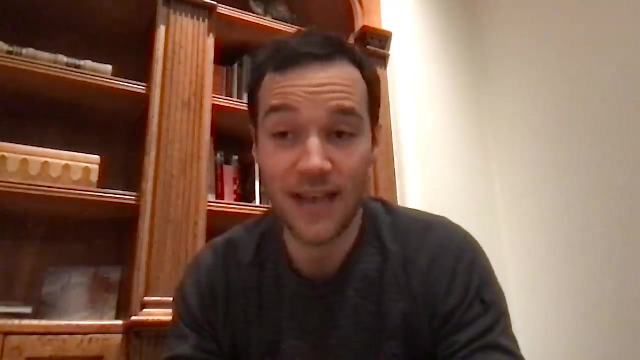 you know, a group just basically proposed a bag of words and led it up to the community to decide how to build on top of that bag of words. that if we put this asset out, the fractal NFT- out to the community and left room for ambiguity around exactly what it could be used for, but sort of 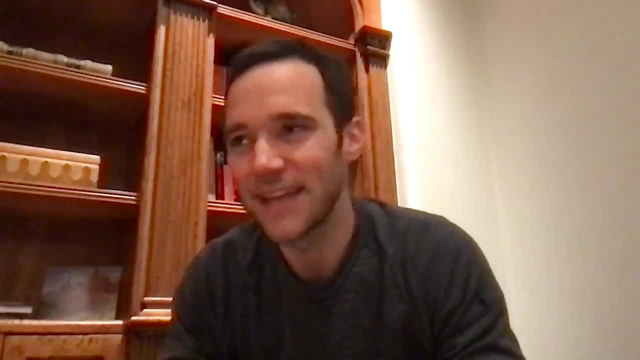 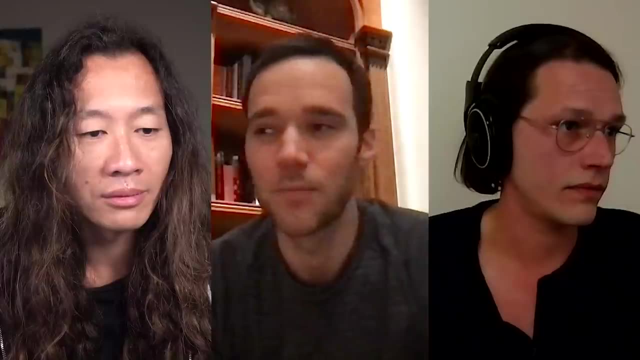 gave hints here and there. it would be really exciting and interesting to see where it goes. And it's been really exciting. I mean it's only been a week or so since the collection dropped, but we're already seeing lots of. we're having lots of interesting conversations around. 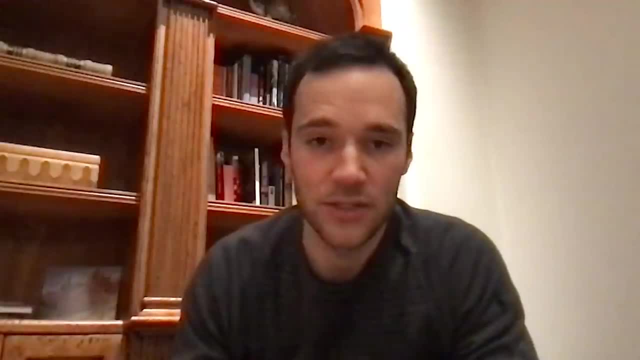 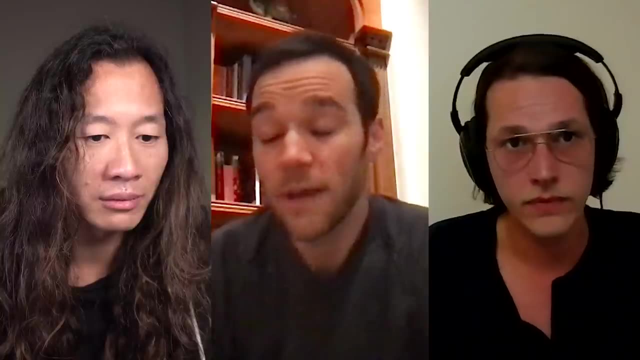 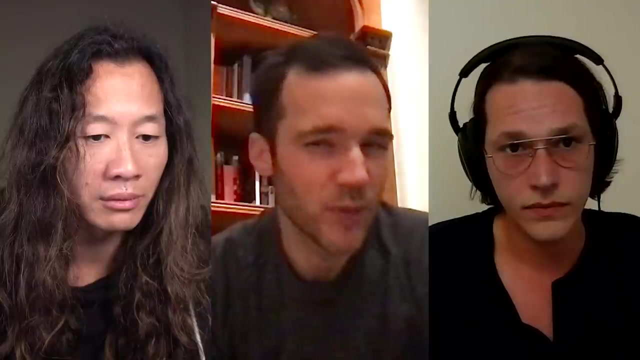 how games think about potentially adding the you know- any utility into their game, Or I mean, you know, and it might not even be anything more than cosmetic, but still there's a lot of interesting behaviors we can potentially unlock with this collection, And 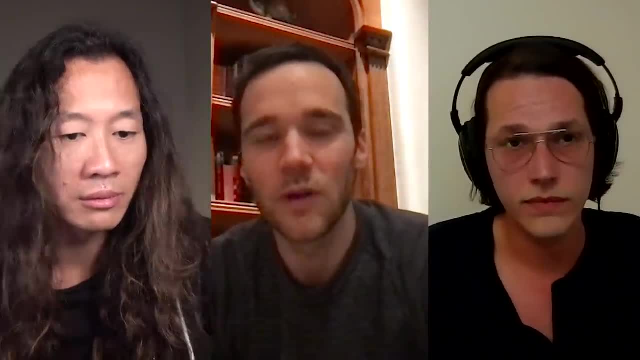 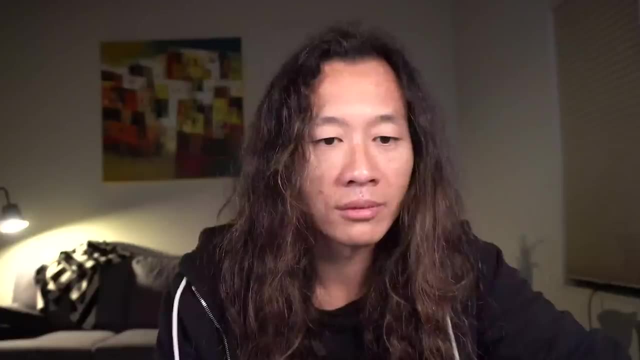 it came together super quickly. We're really pleased with how it landed And we can't wait to see where we take it from here, you know. So one of the things is that it's interesting how it evolved over time for me, because we started 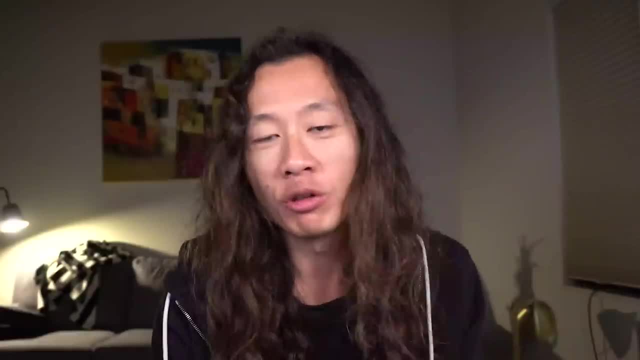 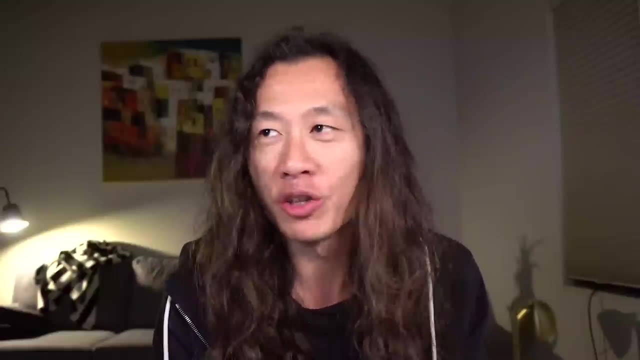 off as like, like you said, it's like a token of appreciation, no pun intended. We're like: let's just drop something, We're going to make it the biggest airdrop, And I really thought it was like: okay, we're investing this, all this Solana, just to like for the lulz, and we'll like distribute. 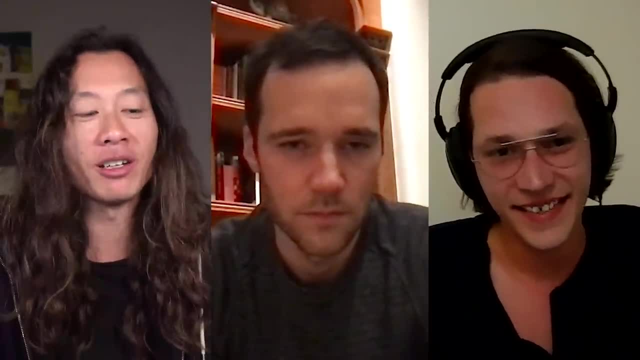 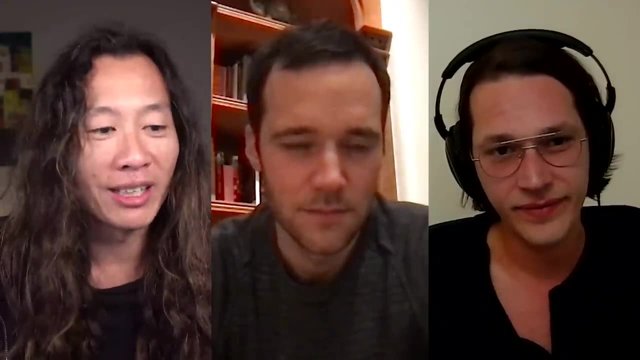 it to people And I really. it's funny because I was, you know, the kind of the one originally trying to pitch- oh yeah, you'll use assets in one game and then there'll be usable and experiences in other games. But you were the one who was like, hey, we had the opportunity to make. 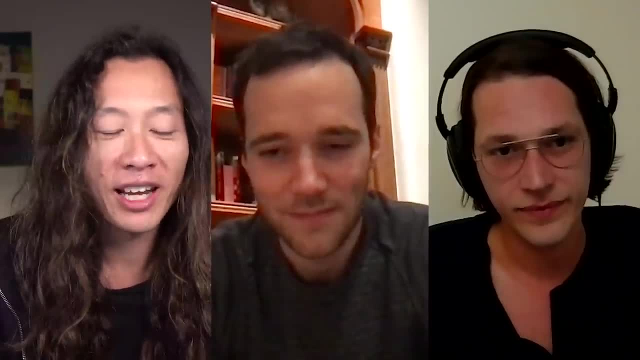 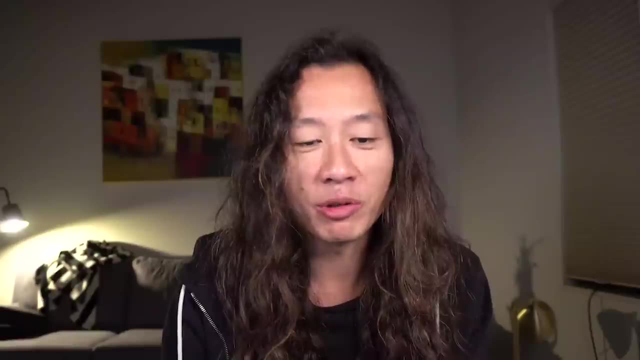 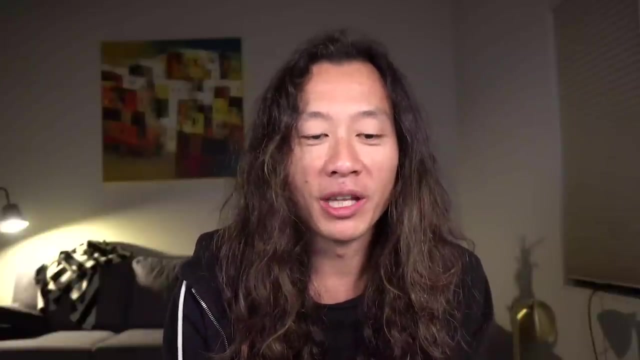 this a possibility right now, And I remember, like you know, everyone was busy. We're trying to launch the site and we had 10 days until we were going to launch it. We agreed to launch it on Christmas Eve, which ultimately didn't happen. We delayed till New Year's, but you were like: 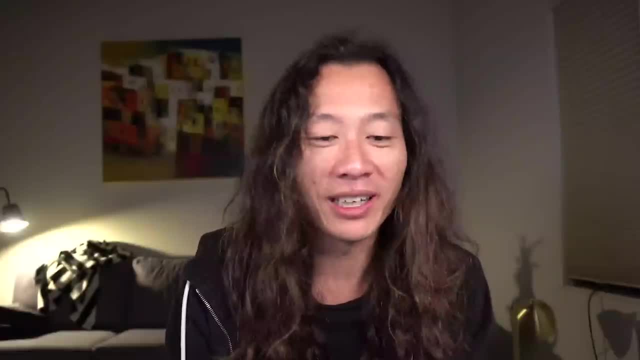 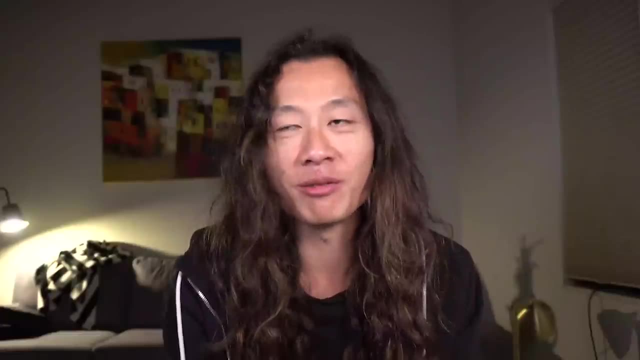 let's spending all this time on the NFTM, like on making, you know, trying to make it awesome and adding all these attributes, and like making the rare, you know, distributed in a certain way, with all the like attributes, And I was like, why are we? I was thinking to myself, like 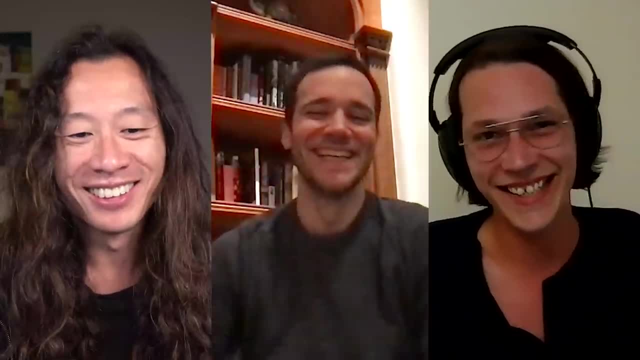 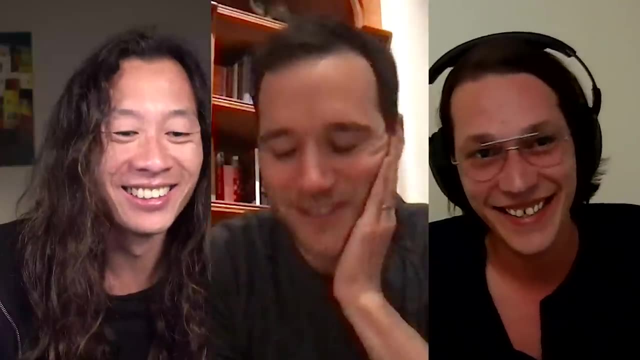 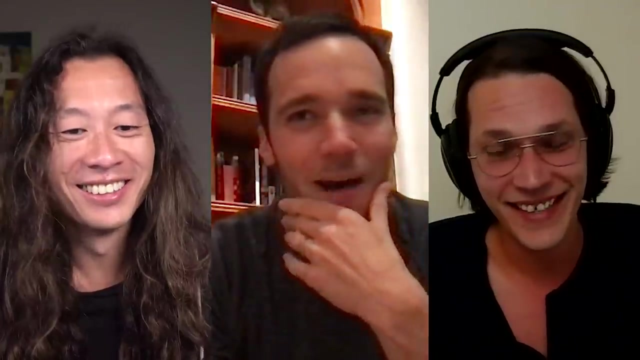 why are we spending all this time doing this? Yeah, I mean, I definitely felt that Robin Robin, one of the co-founders of Fractal, I think, had the same concerns, And thank you for trusting me, Justin and Robin. Yeah, So so how did it like? tell me about the? 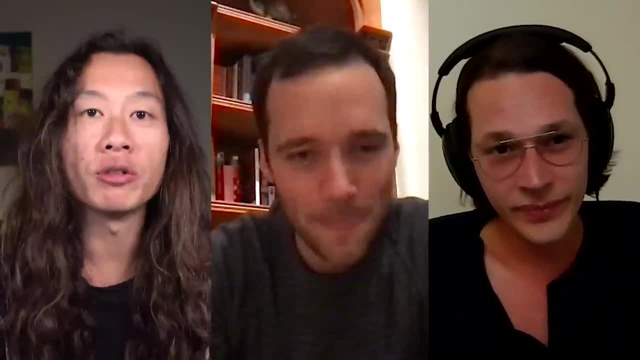 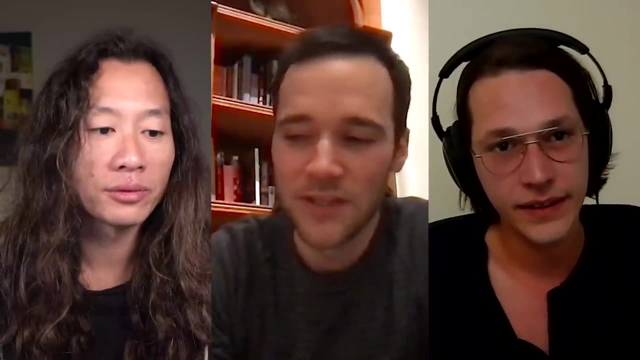 process of, like, all the work that went into it behind the scenes, Yeah, Well. well, I mean first of all- and we'll get into Ludovic's role in this- but we couldn't have done it without Ludovic. He was, he was really critical, And so when you're thinking about, you know, building an 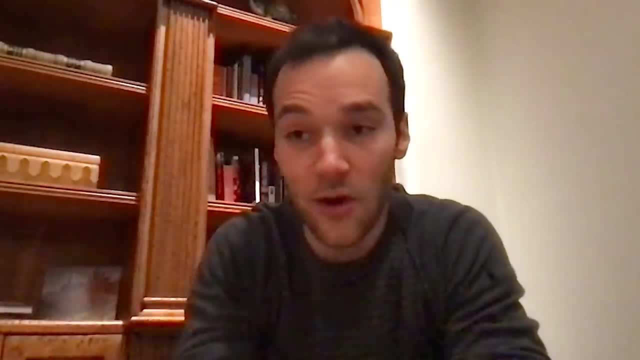 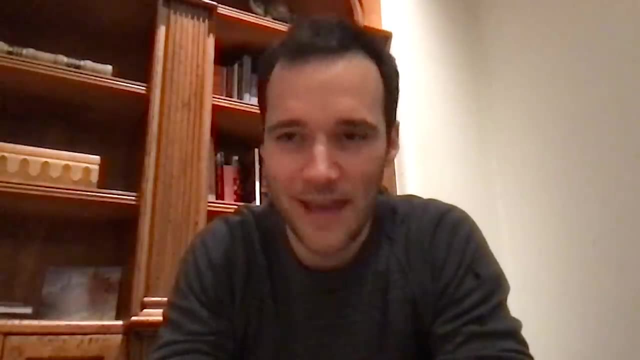 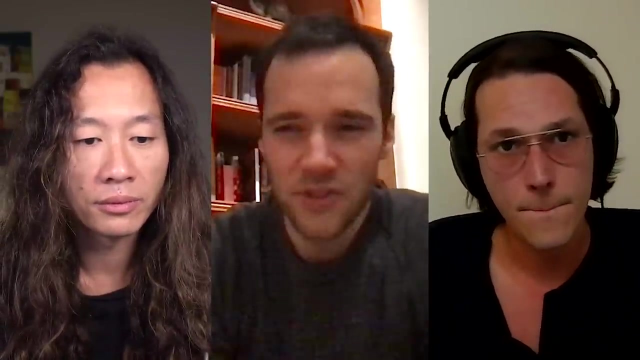 NFT project. I mean, the first step is you have to get the art right And generate the art to be and like we could have pushed a placeholder, but that would have been lame, you know, if everyone's NFT looked exactly the same And also like our emote. our official emoji for the community was a. 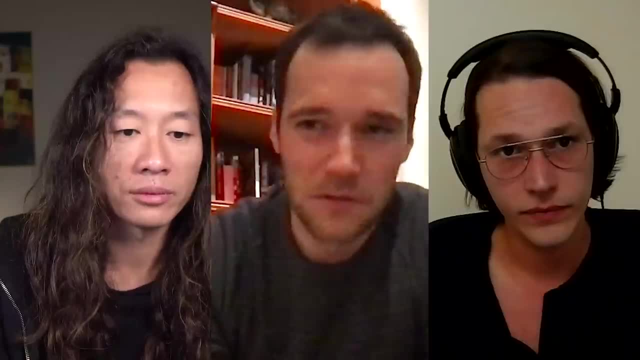 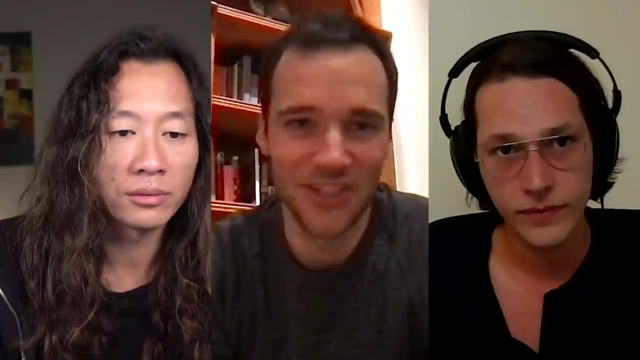 snowflake. Like it's a cliche to say that, like all snowflakes are unique, right, And so we're. like we got to figure out how to pull that off. Like every member of our community should get a. 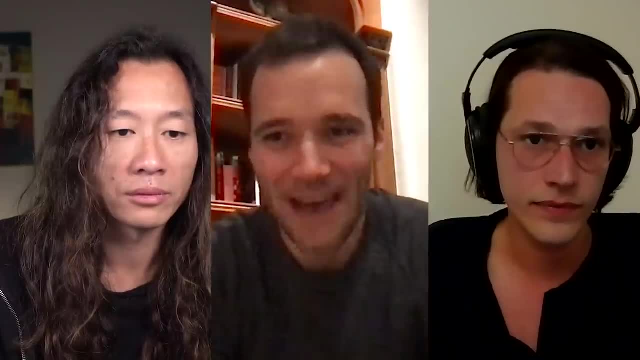 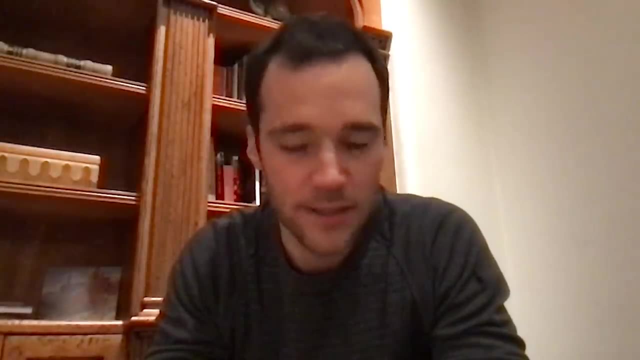 unique snowflake. Like we have to do it. You know, we have to achieve it. We had 10 days, So I mean the first, the very first thing we did was we just needed to find the artist. We got really lucky: We didn't have any. 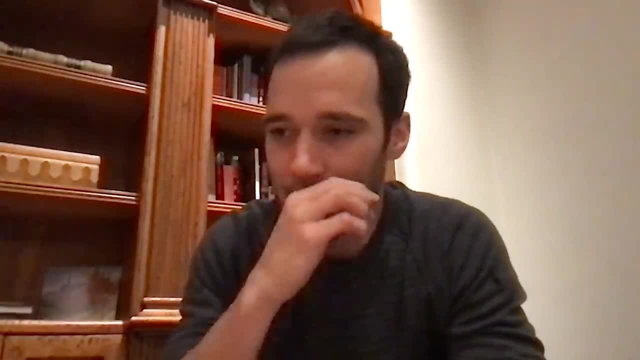 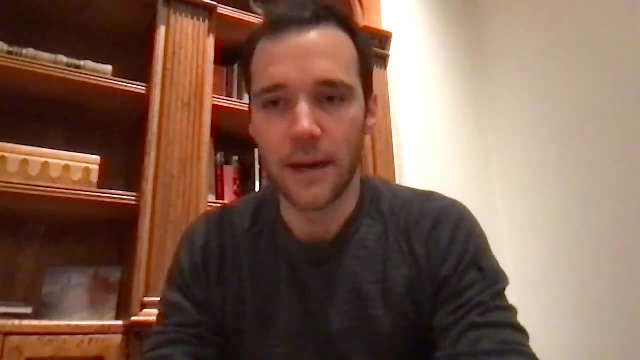 time to get it wrong. you know, I basically I found an artist out of Japan who had done similar work to what we sort of wanted to convey, And actually he was just about- and, by the way, we're going to do a medium blog. 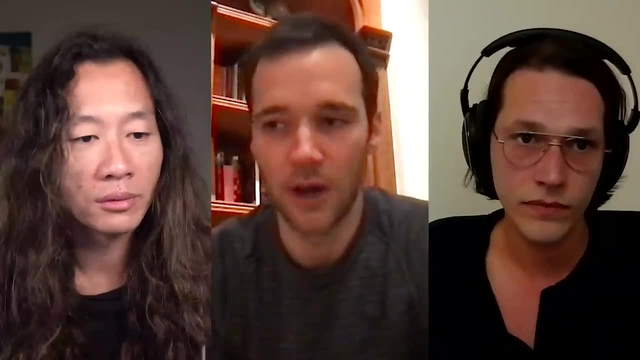 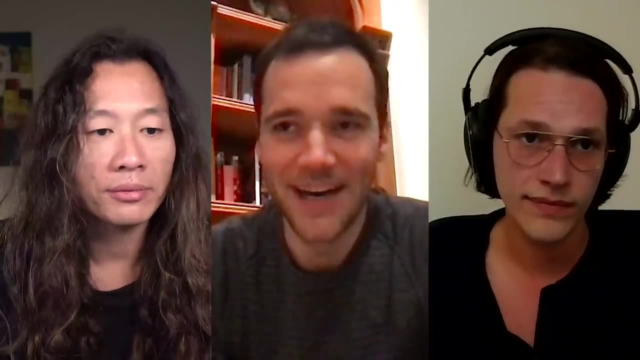 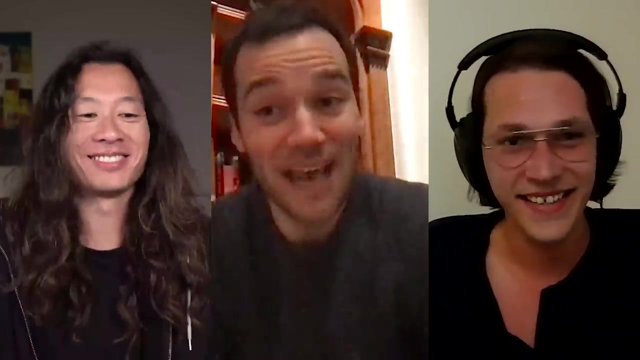 post interview with him. He doesn't speak good English, but it'd be awesome to share his story. he was just about to leave for the holiday break. uh, it was. i mean, launching on christmas is like the worst possible time to launch because basically, you know people, it turns out people. 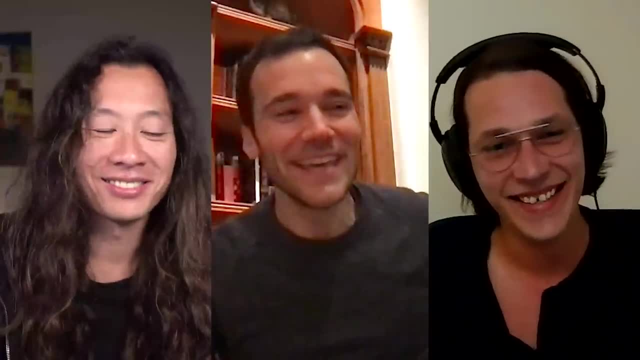 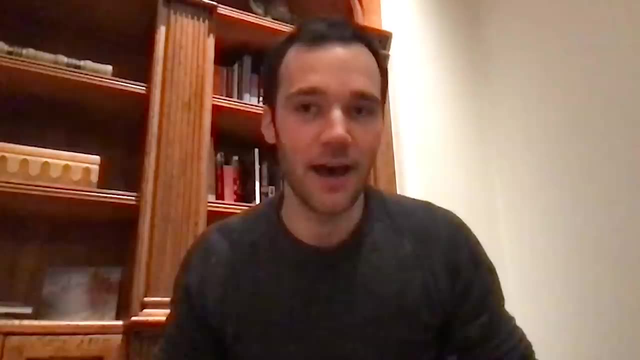 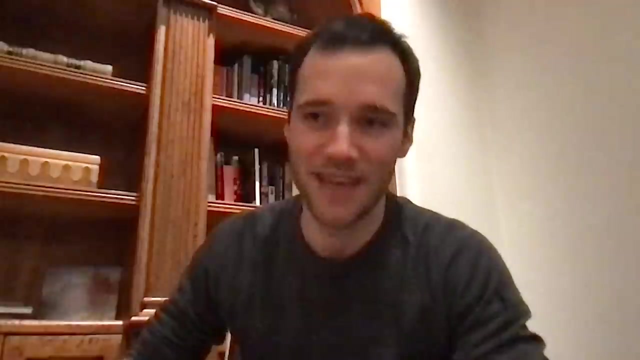 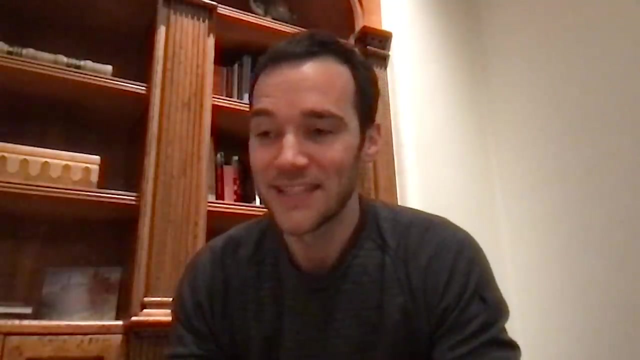 have like things to do. so he, um, he was like we just got so lucky because he was like, he was like: okay, yeah, i, i i'm leaving in like 36 hours. if you, basically if you hire me right now, i will just make it. and he actually had to render the assets, you know. um, so our, our plan was: he, he builds the. 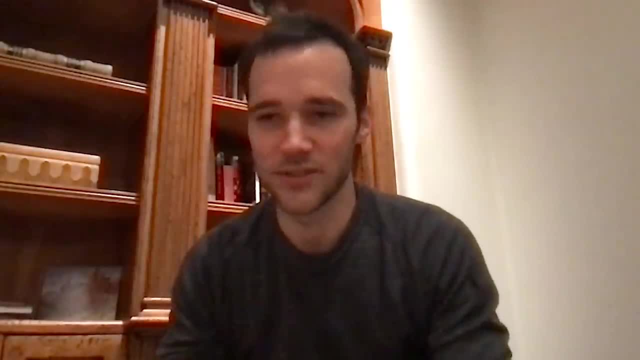 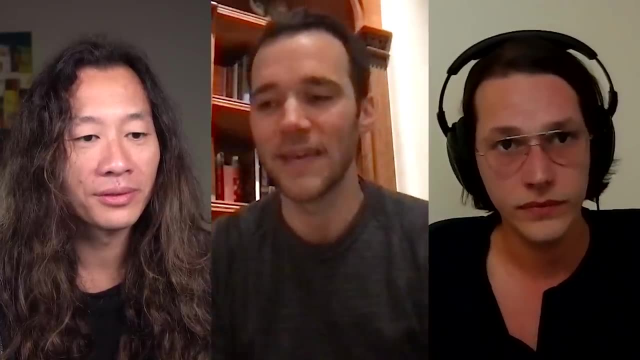 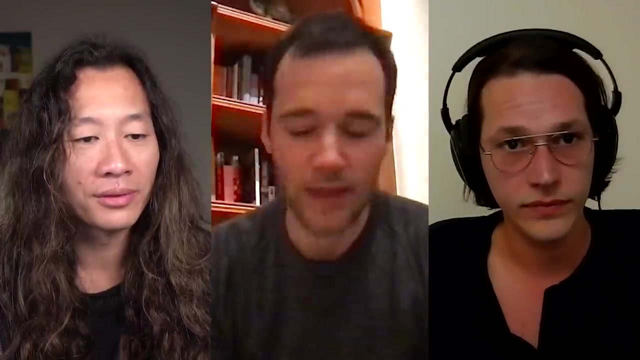 most amazing animations of these, of these, you know, digital snowflakes, and our plan was to just snapshot their, the progression and growth, right, and so he needed to actually spend. i mean, each one of the the renders takes 12 to like 20 hours or something like that, and so he was like doing. 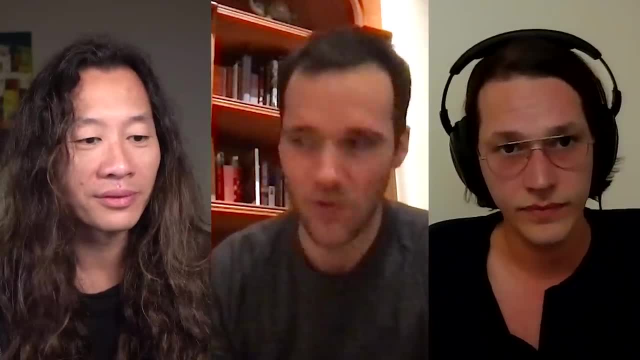 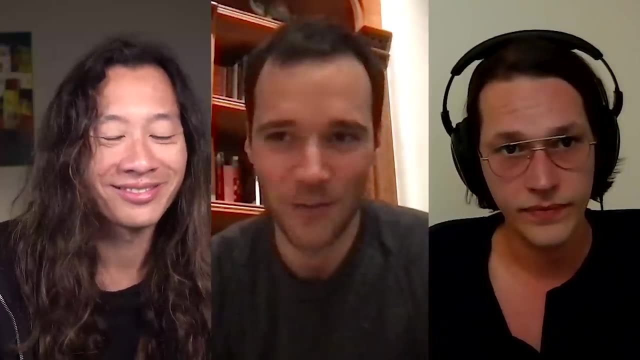 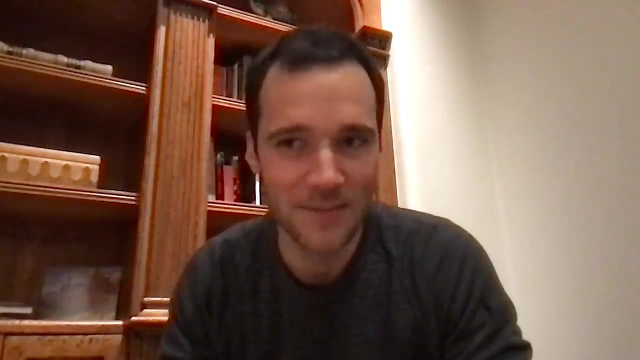 a math about how quickly he'll be able to do the work and spit out the renders so that he can give us the files before he goes on his like 12-day um holiday trip right, where he's not going to have his laptop or anything. i mean, we were i. i was spending some late nights talking uh on his time. 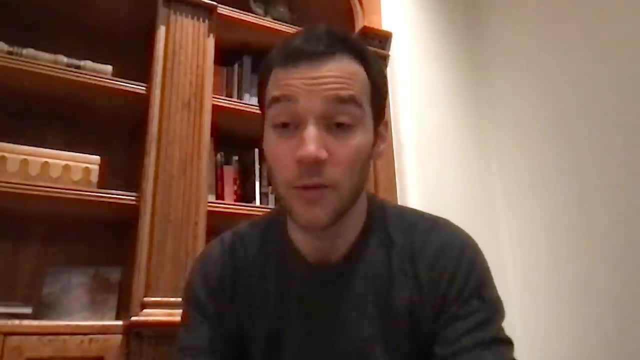 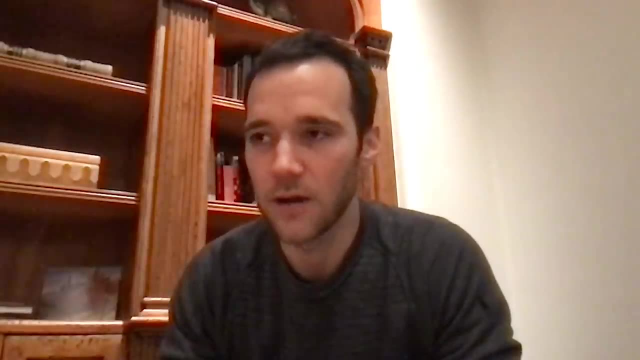 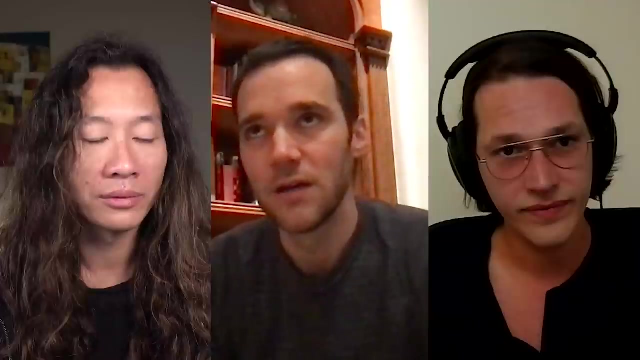 zone, trying to make sure we were going to make it. it was very stressful, but we pulled it off well, at least the first step. but then there was, like, the rest of the project, and this is where his side of the story. so, when you like, when you create an nft collection, you have to plan and 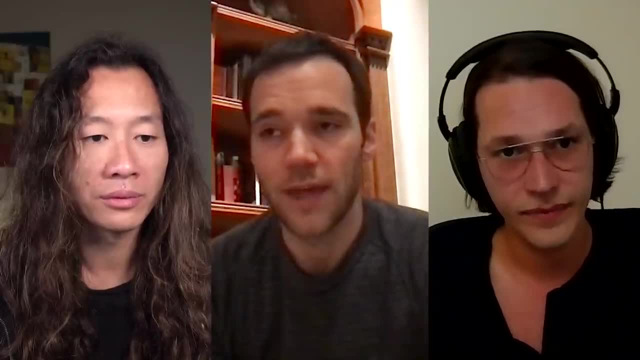 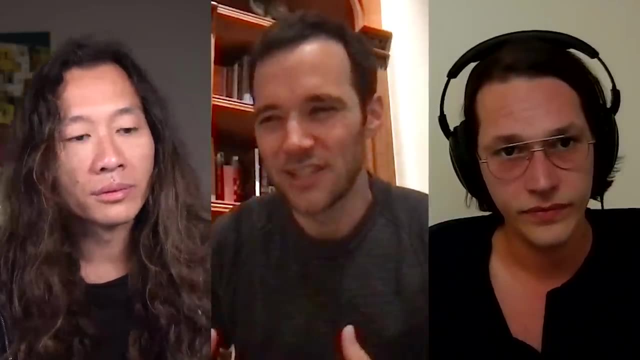 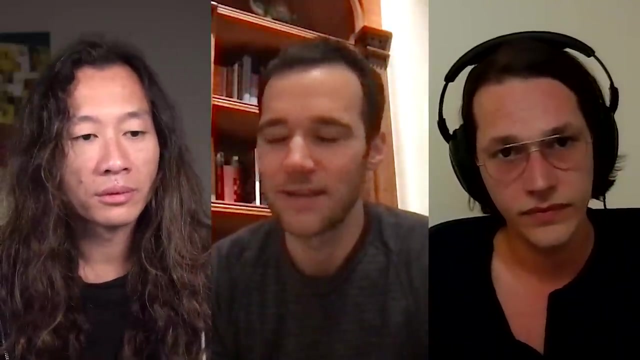 you know the attributes right and you have to make sure that there's, you know, a good balance of all of the rare traits and you want to make sure that the collection isn't dominated by a single trait. there's a lot of things that go into that and so ludic and i have worked together in 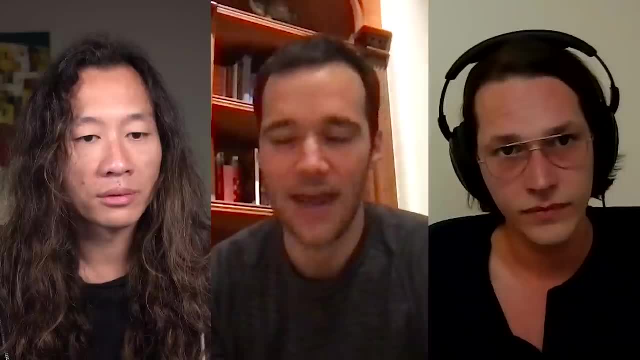 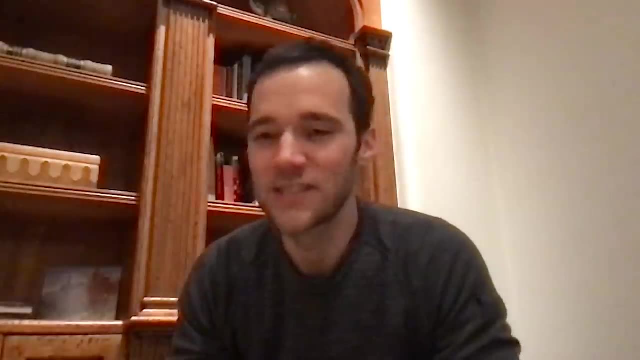 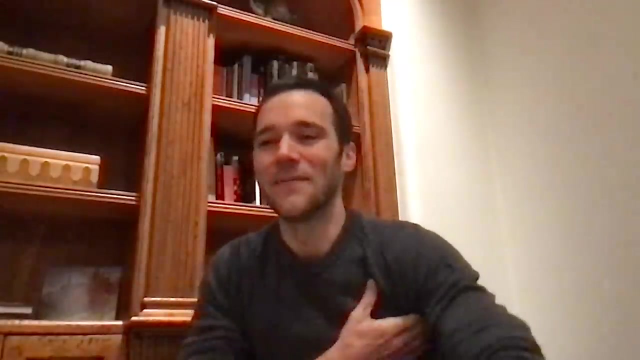 um in other capacities with, like huge data sets, analyzing data sets, trying to pull out signal from noise, understanding root trends. so, like you know it was, it was obvious to me that ludovic was going to be our guy to to plan the um, to plan the collection. and um, yeah, ludovic, why don't you? 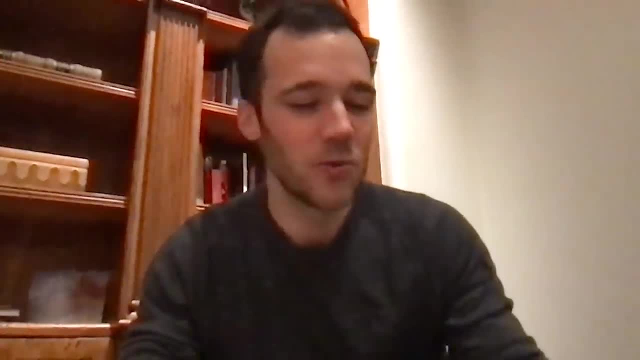 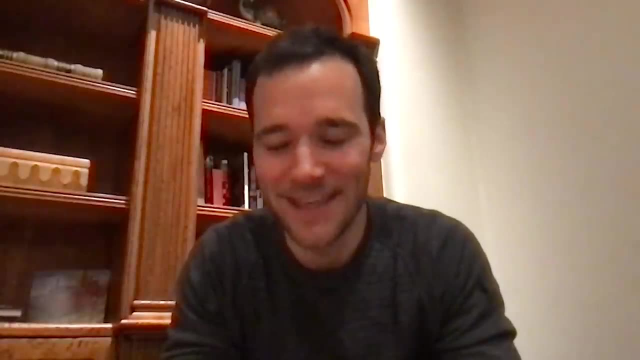 tell us a bit about you know that part of it right, like you, um, you sort of like, took it and and started and started sprinting toward the answer and it was awesome to see it come together so quickly and it'd be awesome to hear some of that story. yeah, well, the the the first part. 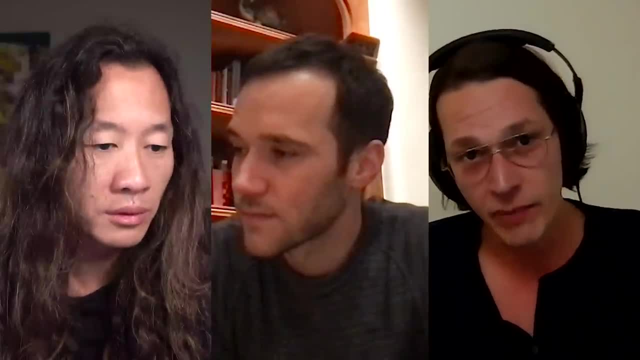 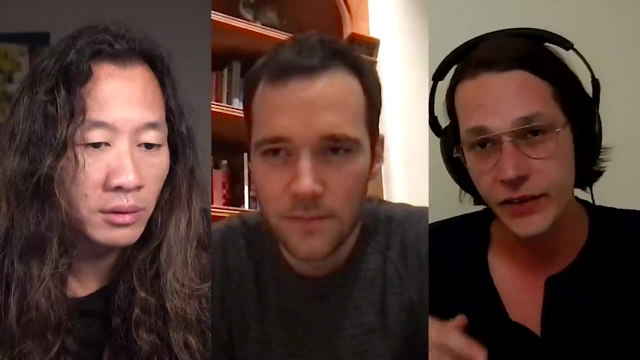 is, we were. we kept talking about that airdrop of snowflakes and their airdrop of snowflakes, so we had to design a bunch of attributes to give to each of those snowflakes and the first thing that came to mind was: this is a metaverse thing, and if we have a whole bunch of 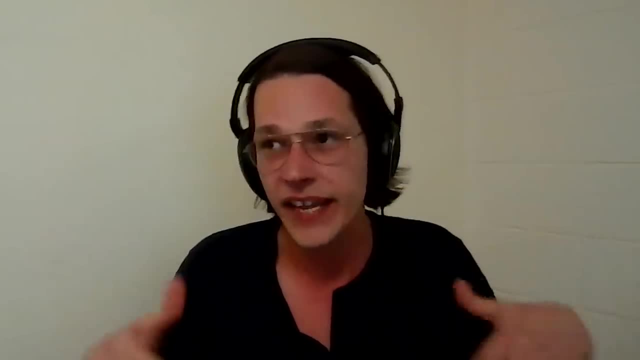 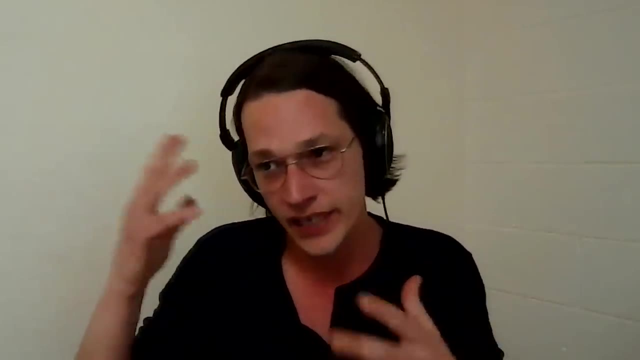 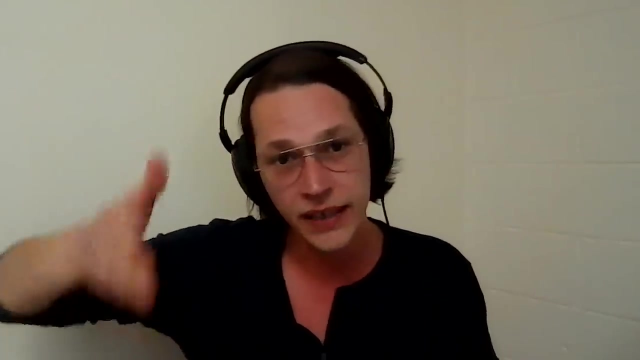 people in game waiting for their airdrop, then the snowflakes would literally come, like fall down the sky, right so? so that's how we. we started picturing the attributes, so like the: the snowflake is at a certain altitude and then it's falling down at a certain speed and as 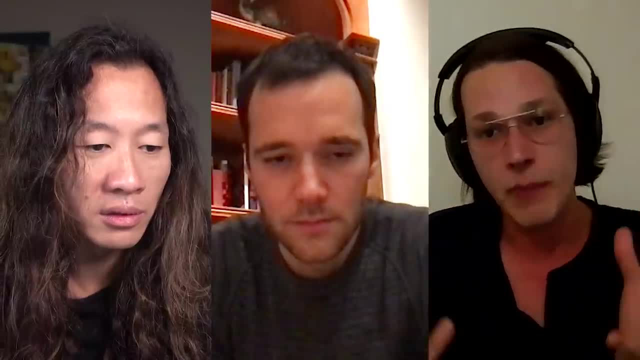 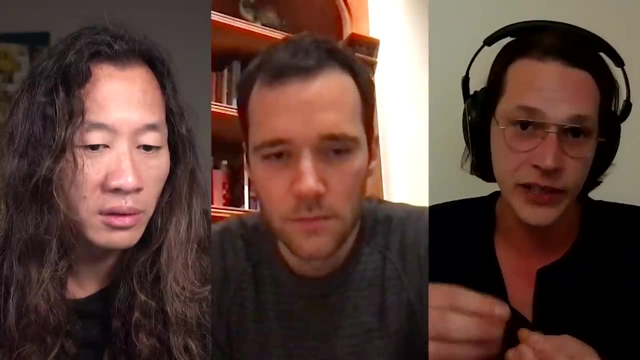 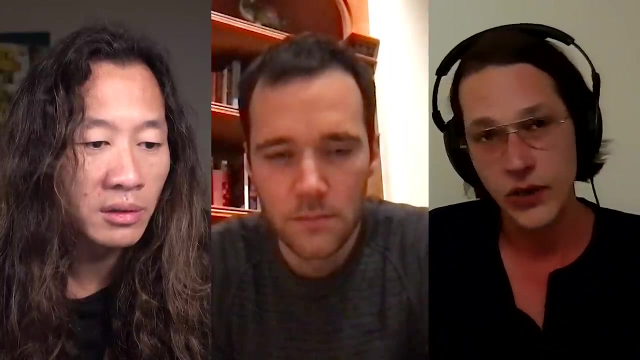 it falls down, it spins on itself and it has a certain amount of power. and and since it's, it's a snowflake, and a snowflake is a crystal. a crystal is made of molecules and those molecules can be very pure or not. so as the crystal grow, uh, you can have a different level of purity. so we- i started- 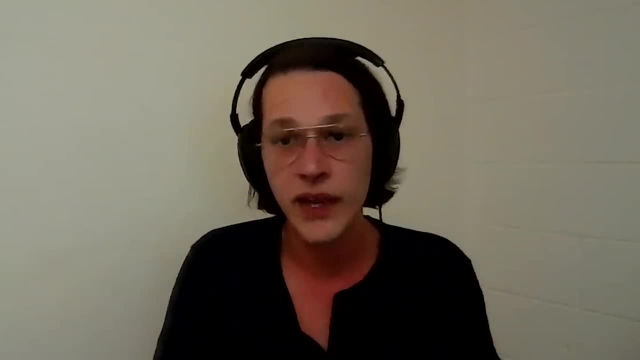 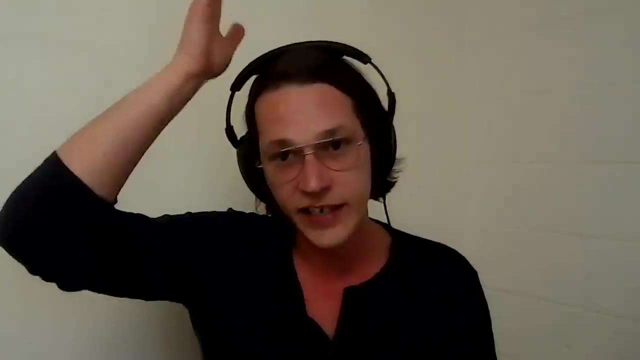 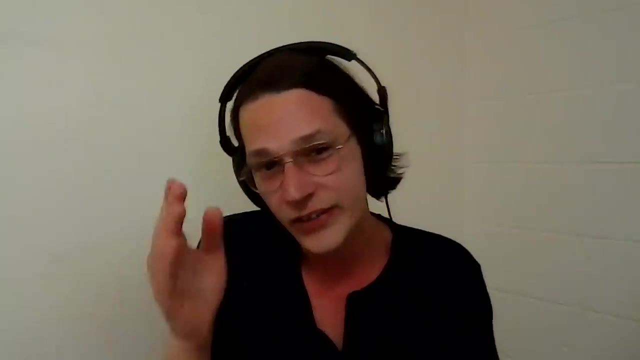 like imagining the distribution for all those quantities and and also started uh putting some uh kind of an easter egg quantity in there, because as the, as the snowflake fall down, you you have a distribution of velocity for uh all the snowflakes and you have a few snowflakes. 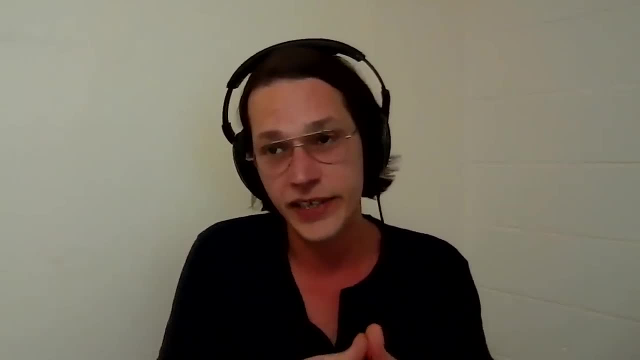 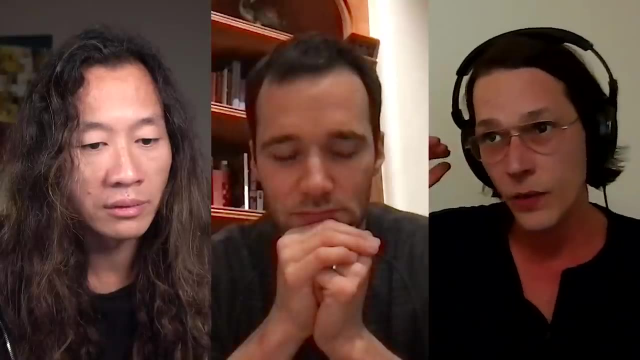 that are over the speed of sound and there is a and there's a non-phenomenon, and if you've seen like military airplane in the sky, you've probably heard that when, um, when a plane goes over to the speed of sound, it makes what what's called a sonic boom. so i i 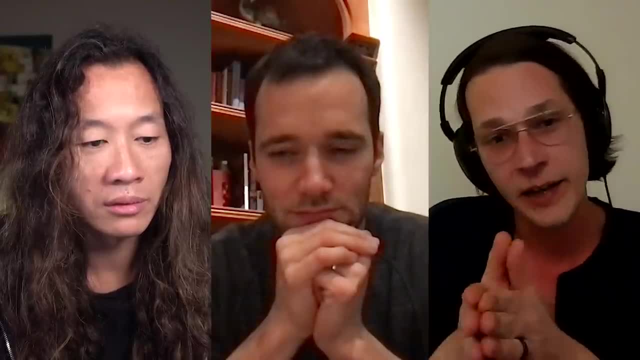 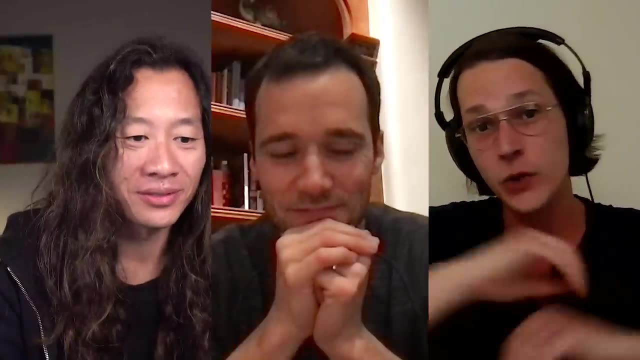 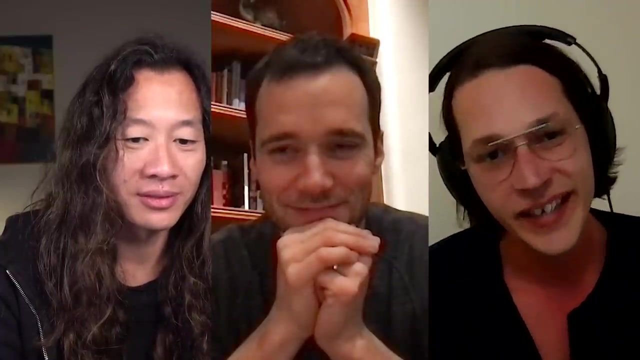 uh, because of- i won't rhyme it whole on that, but basically, as as the, as the snowflake would fall down, this guy, a supersonic snowflake- would make a huge boom in the sky, and so everyone would know someone got a rare snowflake dropped down, uh, from the sky. so that was kind of the i don't, i don't. 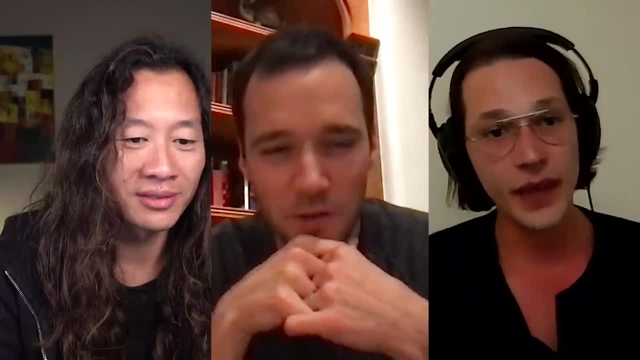 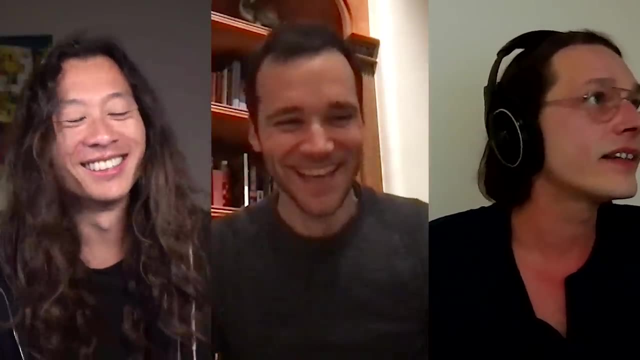 even know the answer to this and maybe, maybe you don't want to share it, but how many snowflakes are supersonic? i can tell you that right now, if you want. so, um, so, while he's doing that, like the, the we're not actually just. 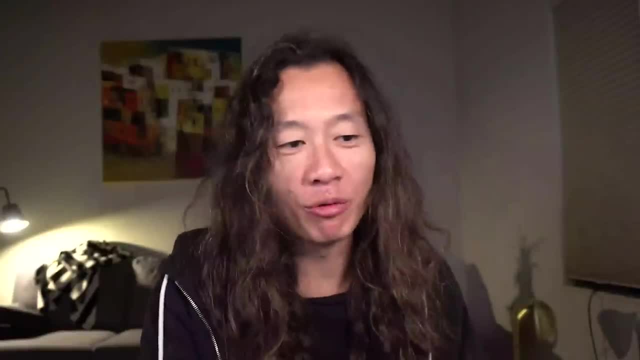 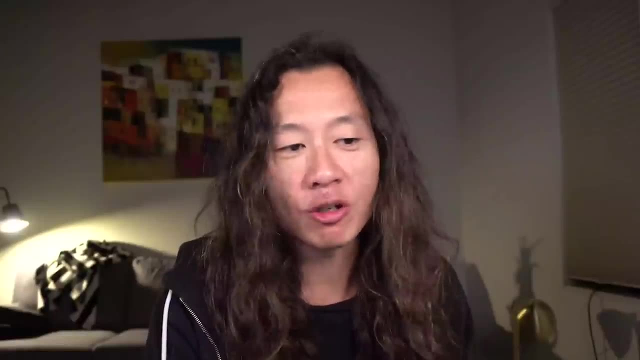 like we didn't just rand, you know, like in each each attribute, like pick a random number for it, like we wanted to achieve certain distributions, like how do we think about? why is it so complicated? yeah, okay, so there's, there's a few things, uh, okay, so now just to answer the question. there's a 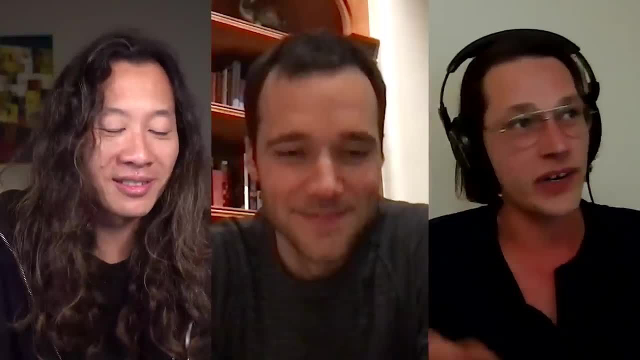 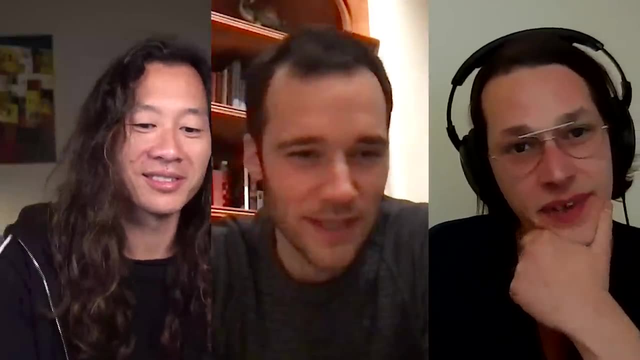 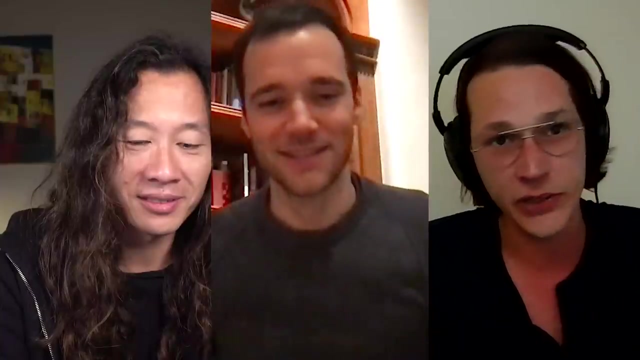 a little bit over 2 000 supersonic snowflakes. uh, over the hundred thousand. all right, so, and people need to google the speed of sound. i guess the velocities and meters, uh per second squared right, right, yeah, all this is in physicist unit. so, uh, purity is a pure number, altitude is a meter. 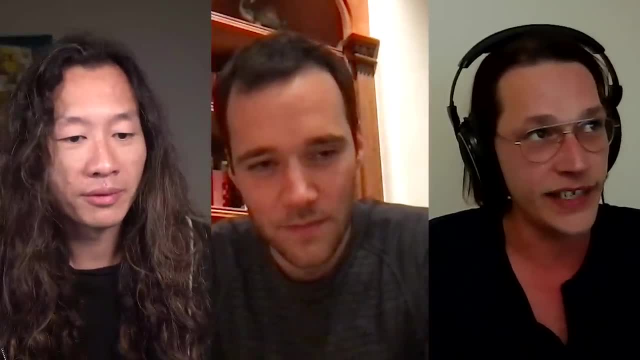 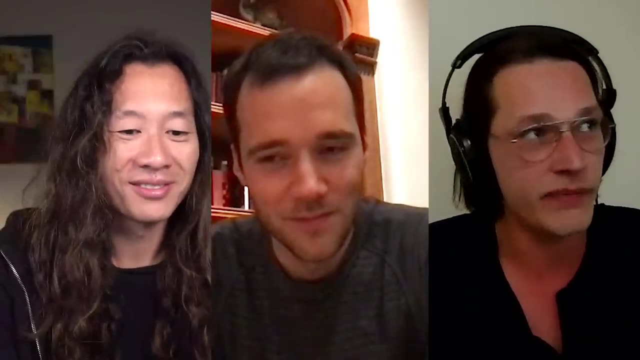 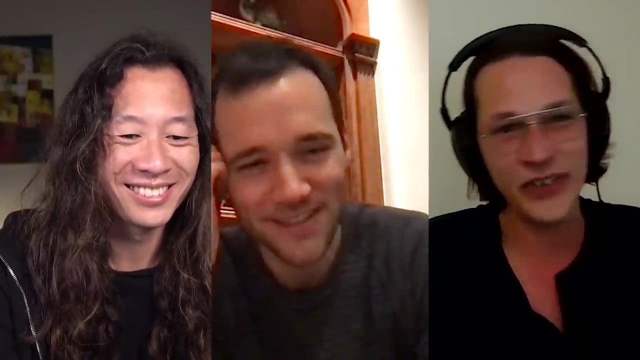 the, the spin is in degrees per second, velocity meter per second and power? well then, you figure it out, because power is not exactly a physicist concept. it's not in, it's not in kilojoules or something. yeah well, the scale from zero to a hundred, where, well, 20 to 100 doesn't make quite as much sense, but uh, yeah. 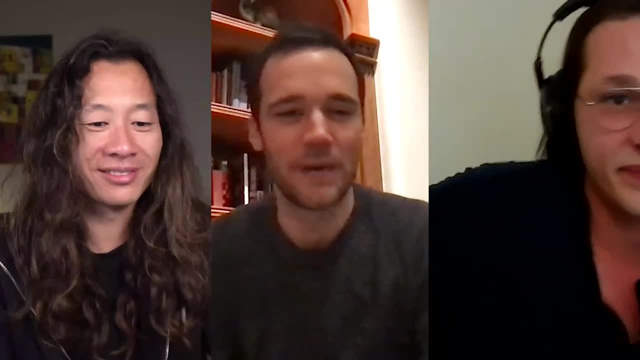 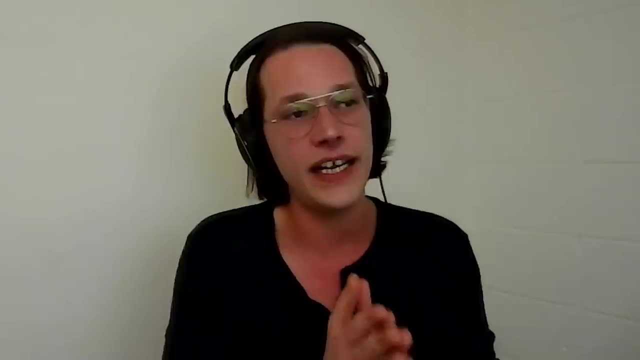 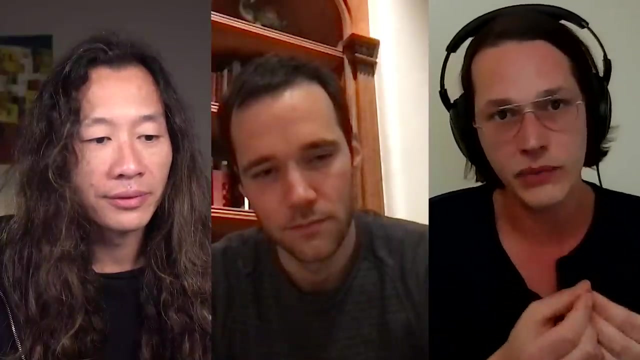 yeah, it's sort of like a stickers bar for a full powered rectal. so so, yeah, we, so the distribution. what's so complicated about it is trying to give everyone a chance to get a very rare snowflake. uh and uh and and not make so not and uh and uh and not make. so not uh and and uh, so not. so uh, uh and not make some. uh, two like zero so66 village. but uh, uh, this is very, very rare snowflake. uh and uh and uh and not make some about that. uh, the soft side of it is about a 200 scale. 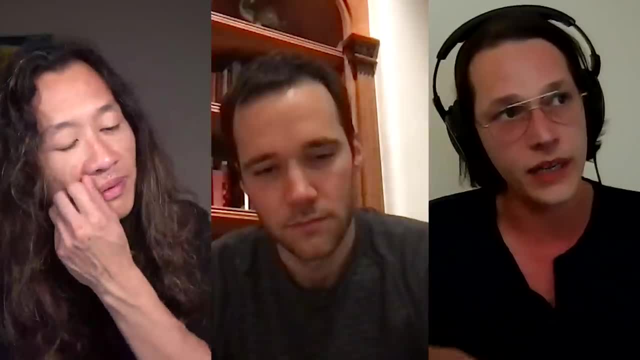 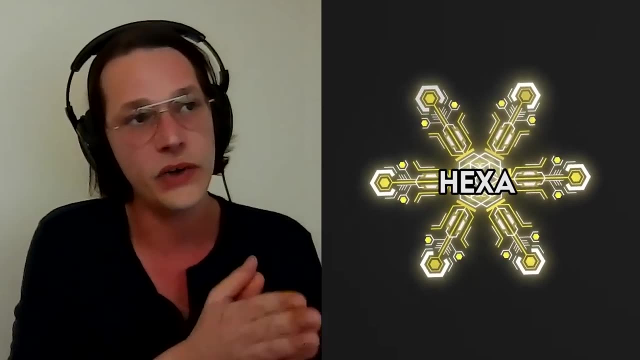 of the same customer'll chop bits. the other true example, someone's with five, Тогда millfieldsen we're. So you have those four factions right, And people that were very early get snowflakes from the exit faction. And so, since they're very early, we wanted to give a little bit of an edge. 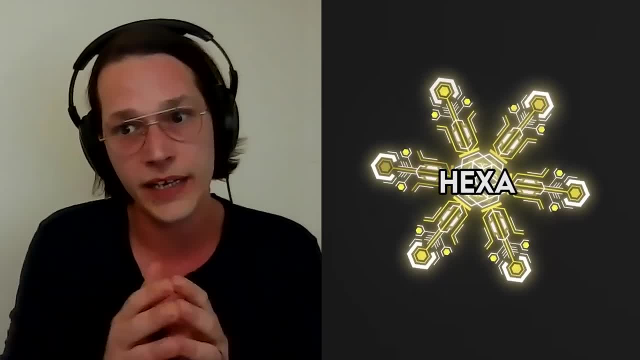 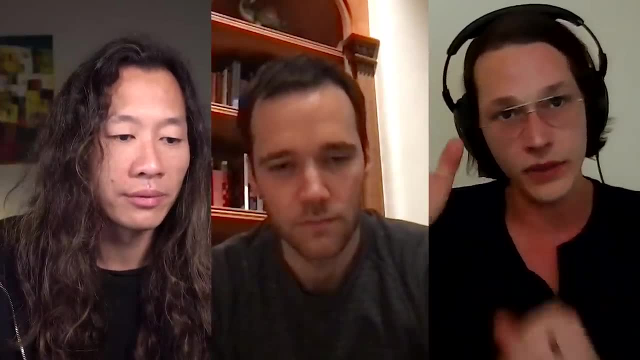 So on average the exit snowflake has higher attributes on each attribute. But as you go down, on average each snowflake is a bit lower. But when you get in a trifaction there are 70,000 snowflakes there. 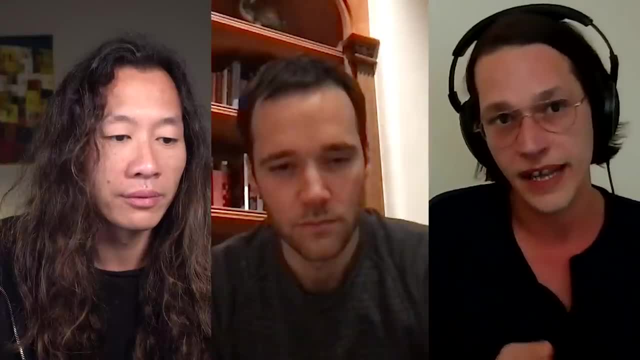 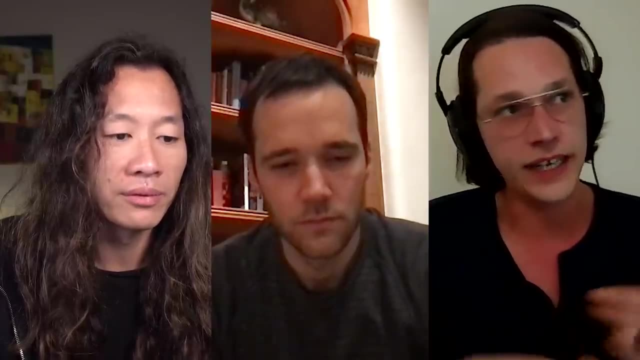 And so you roll the dice more often And, as a result, you get more extreme values, Like in statistics. we call that the black swan effect, Like if you see a bunch of swan and if you see five swan, you'll never see a black swan. 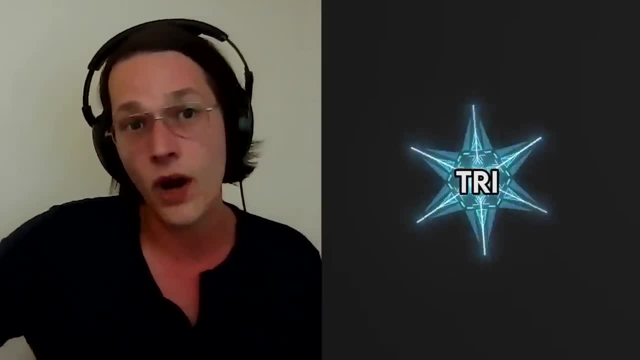 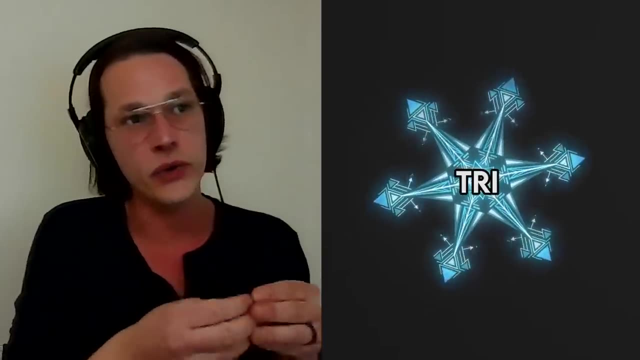 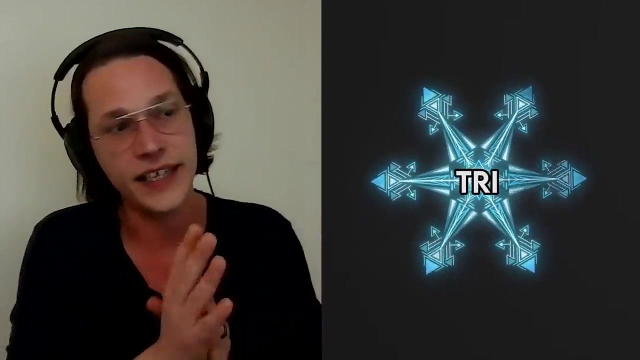 But if you see 100,000 swans, you might end up on one very rare black swan, And that's one thing I try to convey in the distribution here. So you get like very, very rare snowflakes And the trifaction, even though it's the faction that has the least of an edge. basically, 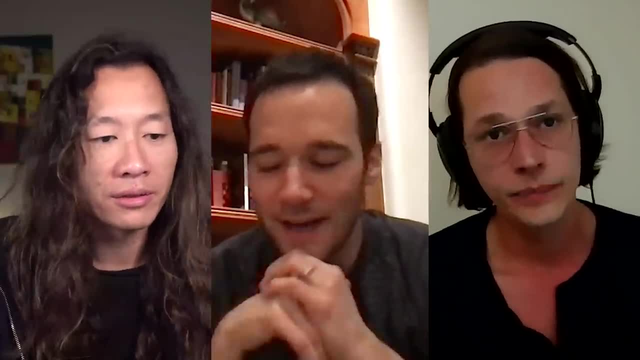 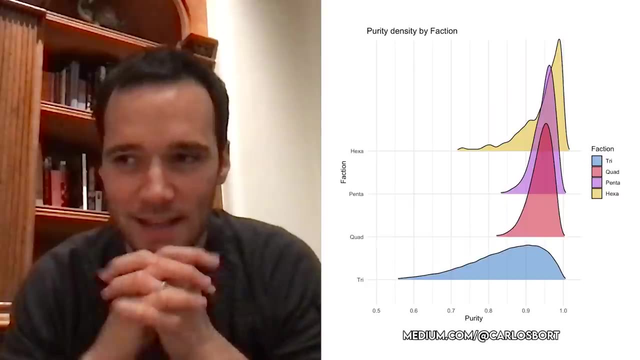 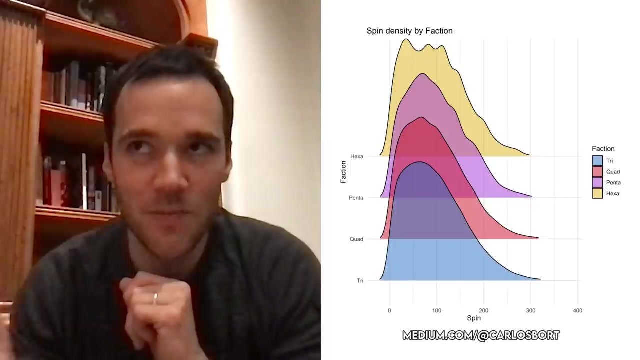 What I love is we had a community member do an analysis of a subsample of like 3,600 fractals And they plotted out the distribution across each faction and such, And it was the first time, I think, the community realized that. 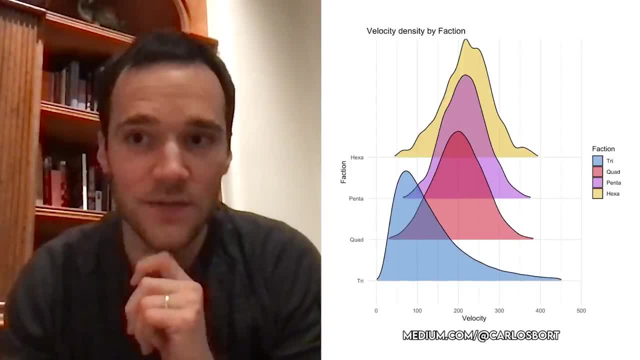 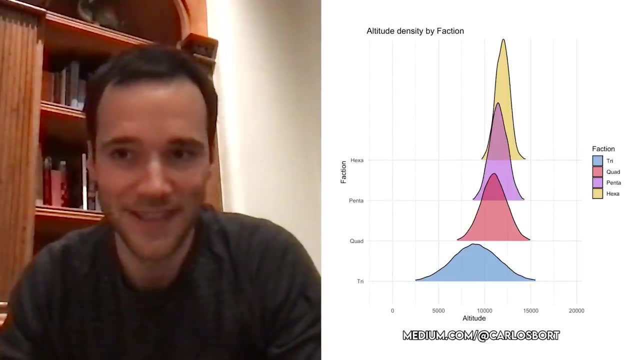 some of the you know, some of, like the tris, for example, and I think the quad and the pentas as well, have some really rare special fractals in there. For exactly that reason. you designed it with that in mind. 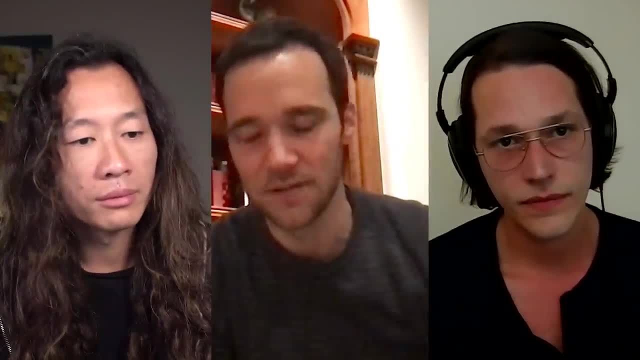 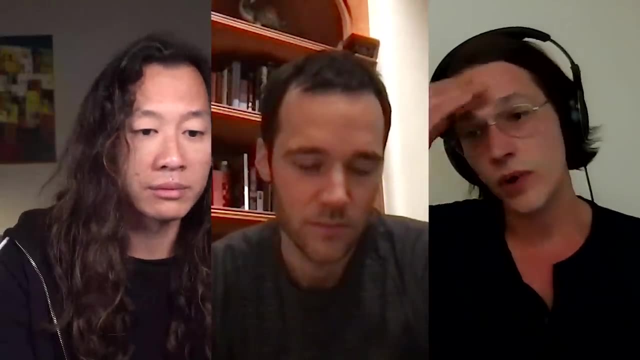 Because we don't want the collection to be dominated just by a single faction, Because there's more to the collection than just the faction attributes. right, Yeah, that's it, And that's one thing that I spend so much time on is calibrating all of this. 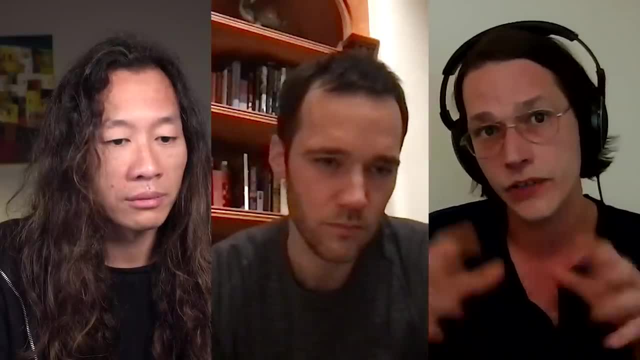 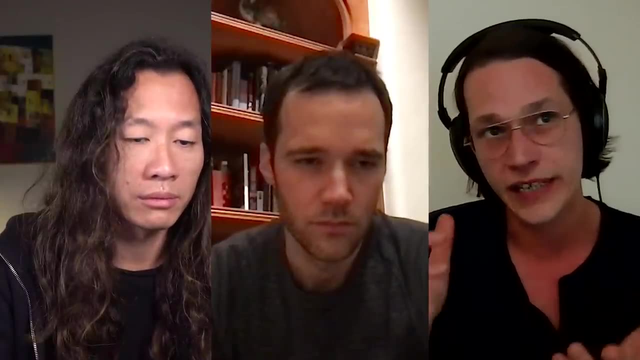 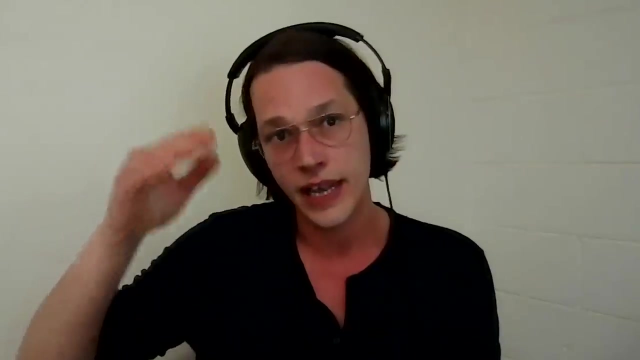 You know, we wanted to have a distribution such that when you look at like the probability to have a certain snowflake, that this like low probability snowflake you could interpret as the rarest snowflakes, And we wanted to make sure it was not completely dominated by exaFaction, and then by quad, and then penta, and then tri. We wanted, like in every slice of rarity, to have a mix and match of all four factions, And so that required a lot of work. Gotcha, Yeah, that makes sense. Yeah, so one of the things we were really interested in is like trying to figure out utility for this fractal right. 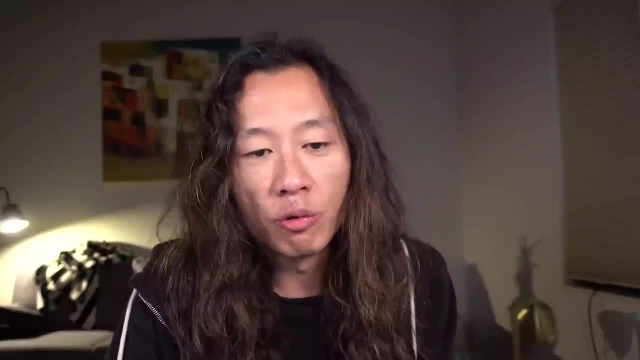 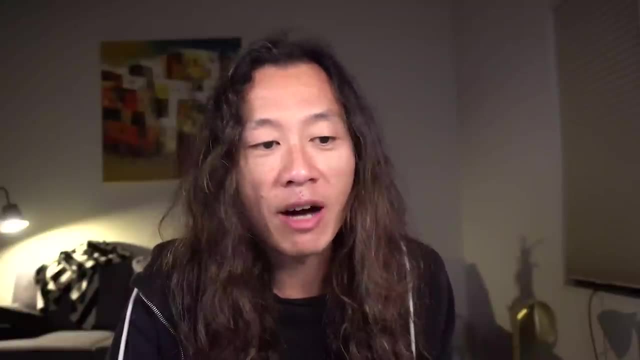 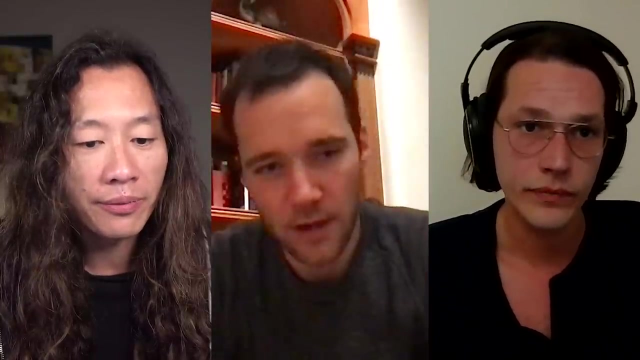 For this fractal collection. So what are some of the things that we're planning on doing on fractal itself in order to drive some value in the fractal for the community? Yeah, I mean to some extent. we're not 100% sure yet- 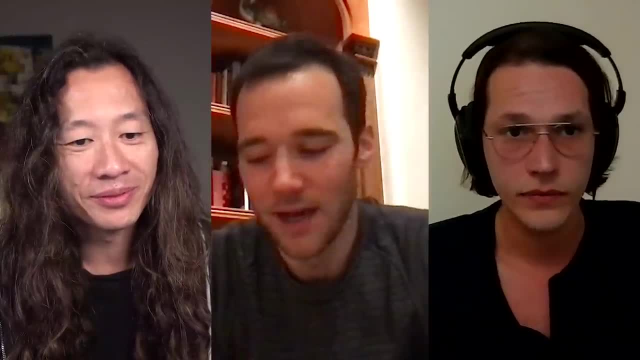 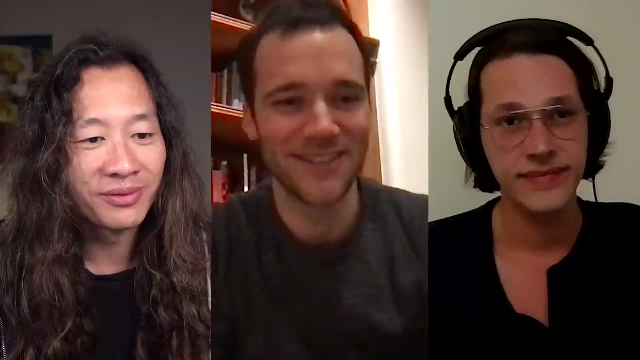 There's lots of really exciting ideas we have, And some of which we'll talk about, but other things we haven't even thought of yet, right? So I don't want this to be considered like the de facto answer to that question. just for the record. 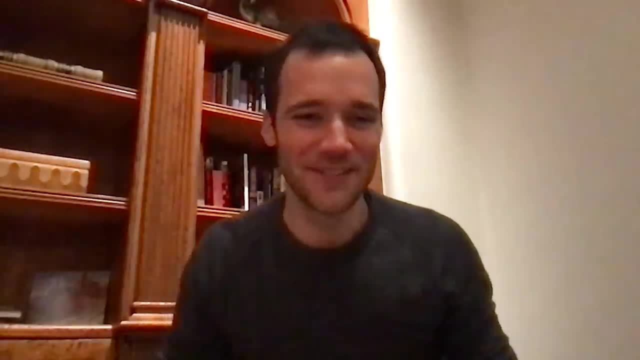 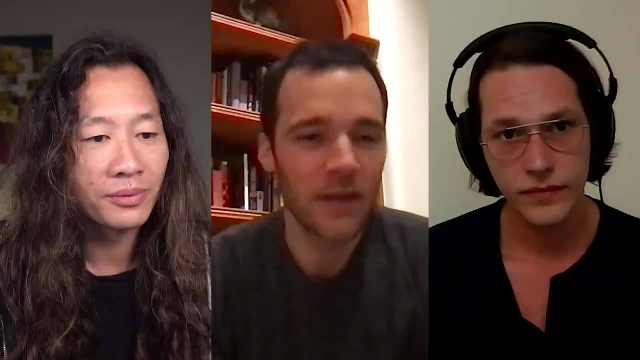 And I mean that because I think we're going to come up with even cooler ideas than what we might even talk about here. So I mean, you know the fractal community, owning a fractal should mean something within the fractal community, right? 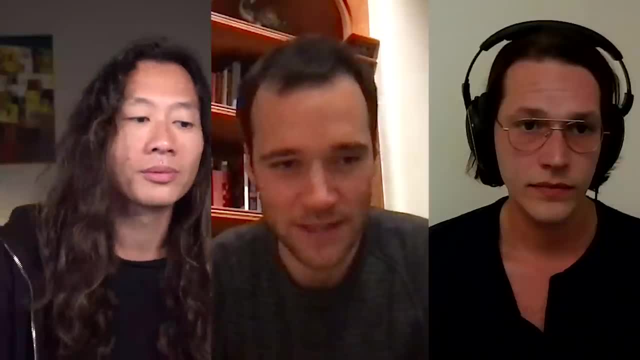 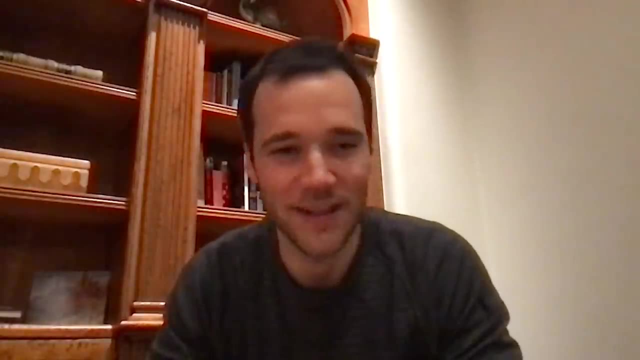 Access to special events, which we actually have some on the calendar now I'm not sure if we've announced them yet, But we're going to bring some special guests to the Discord to have some awesome conversations with the community. And, you know, being able to bring folks on stage for live conversation with the guests would be just like one example of some cool stuff. 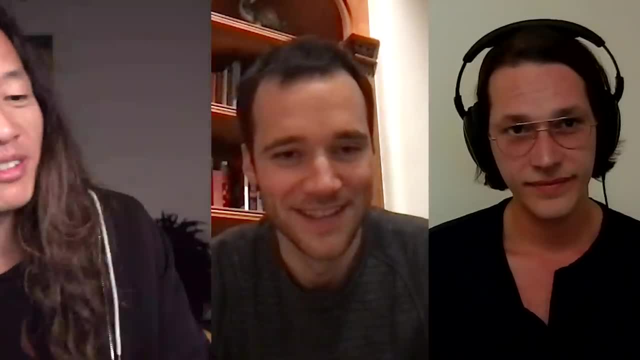 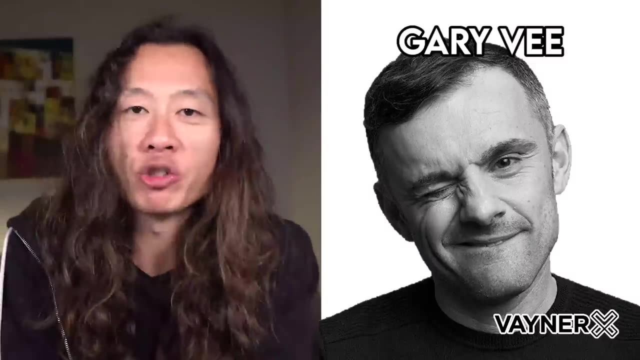 I think we can announce them right, Like I mean, it's going to happen soon, Like we got, let's just do it. We got Gary Vee coming for a special chat with us To our Fractal holders, as well as Emmett, my Twitch co-founder, the CEO of Twitch. 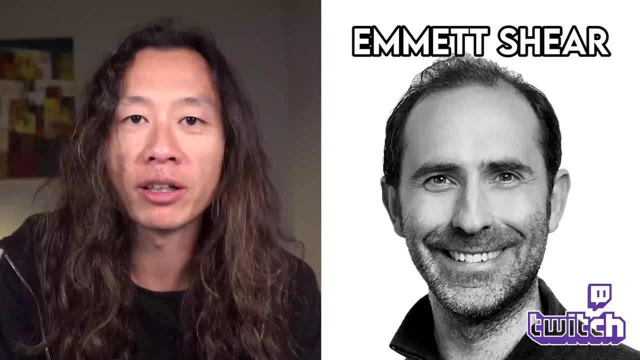 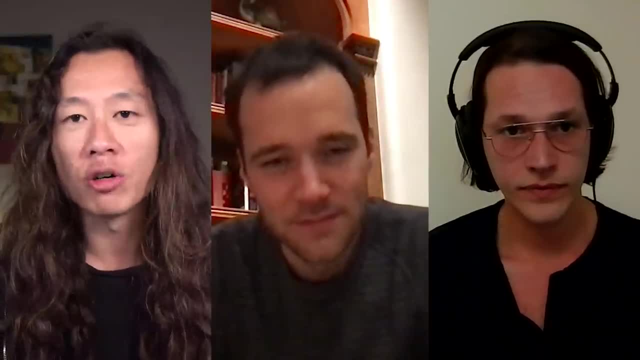 So we'll drop the date soon for when they're going to come. But if you're a Fractal NFT holder, you'll be able to get in that chat and Discord and ask questions to those guests And we're going to bring out more as well. 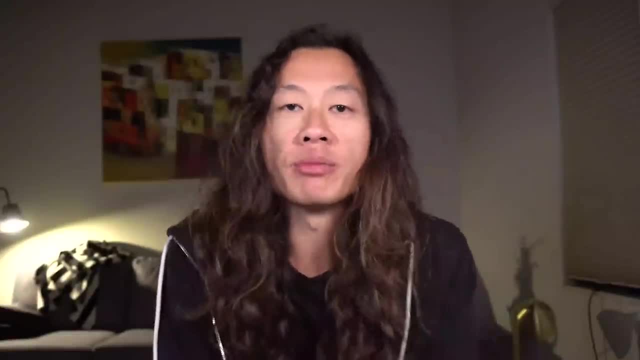 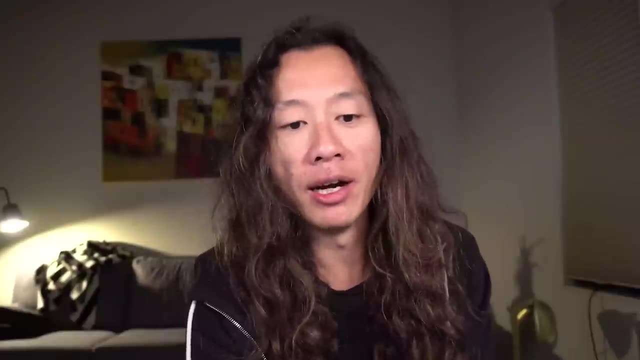 And then the other thing we're planning on doing is obviously there should be some benefit to holding Fractal NFTs with Fractal itself, like with the marketplace itself. So, David, do you want to talk about some of the things that we've talked about there? 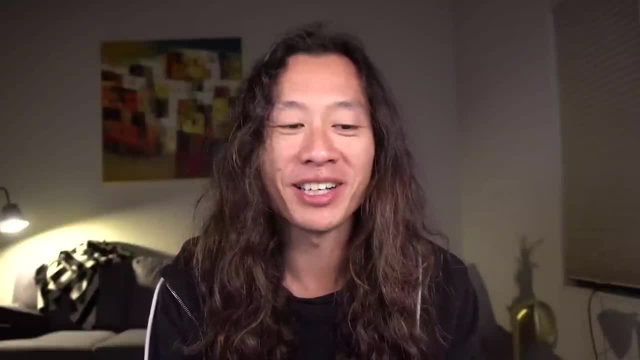 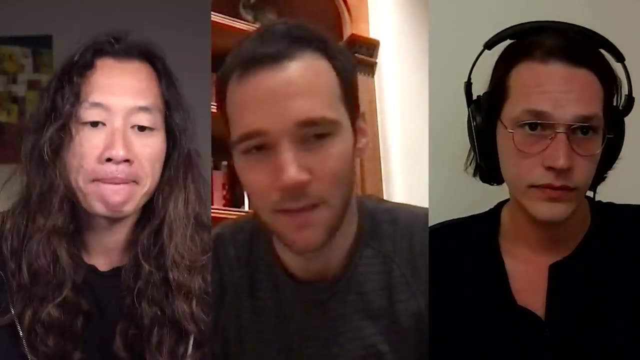 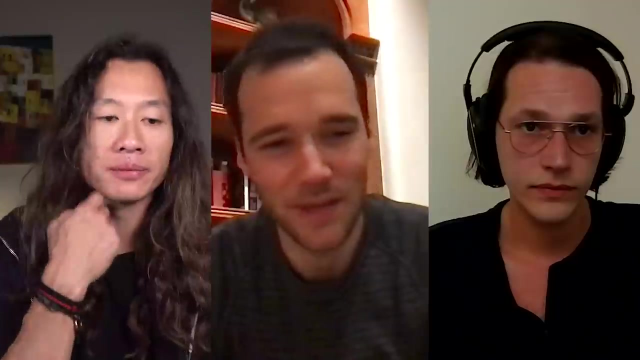 I'm not sure how specifically, because we haven't really decided yet, but we have a bunch of ideas. Yeah, I mean, it might provide some benefit in some mints. If Fractals are held by real people, then it might actually be a really good anti-bot solution, right. 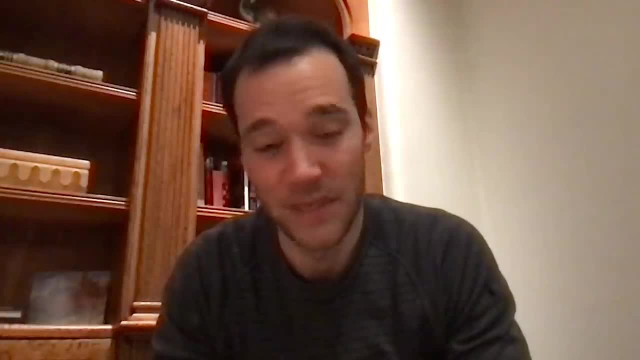 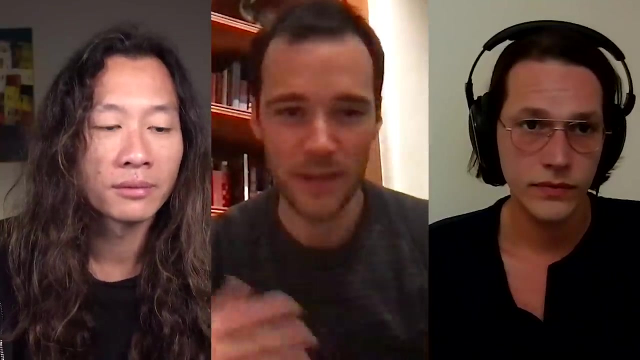 Because there's a known community of folks that would mint a project And so maybe some of these games actually prefer to have the Fractal NFT holders on the whitelist. So there might be something around just access. I think there's probably going to be some type of, you know, some type of I don't want to say discount, but definitely some, you know. maybe there's some economic incentive to participate. 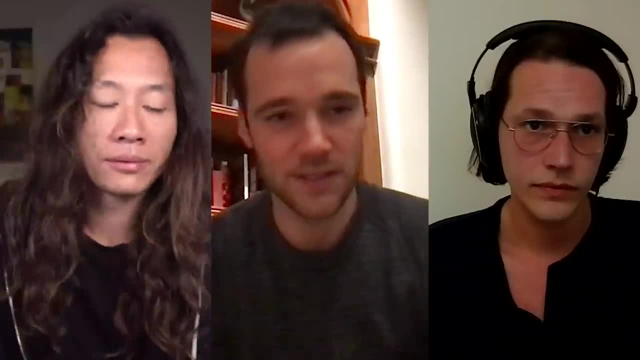 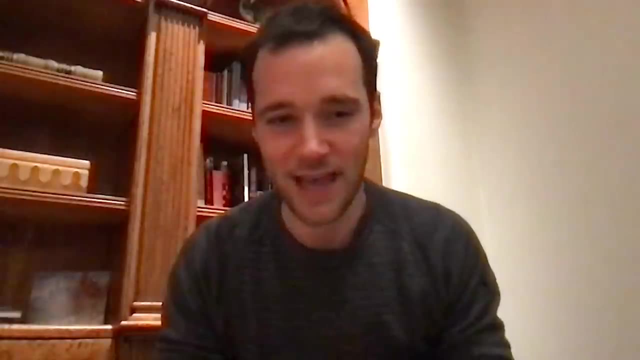 Maybe Fractals are airdropped to folks in the marketplace that are most active buying and selling on Fractals. Yeah, You know, and this is where we're not exactly sure. but you know, Fractals are sort of a way to symbolize who's within our community. 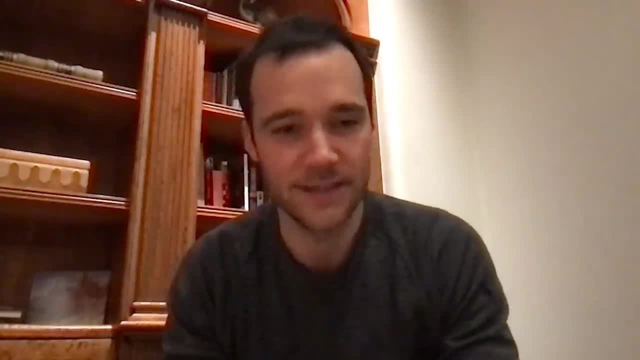 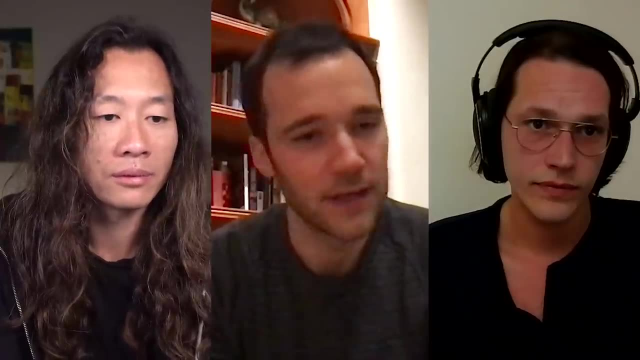 And we want to use it as a way to reward and incentivize the right behaviors within the community, And so you know. so perhaps, like your trading activity and all that stuff could actually unlock Fractals for your wallet in the future. 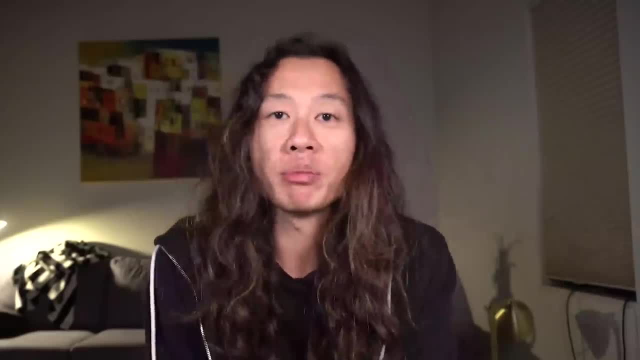 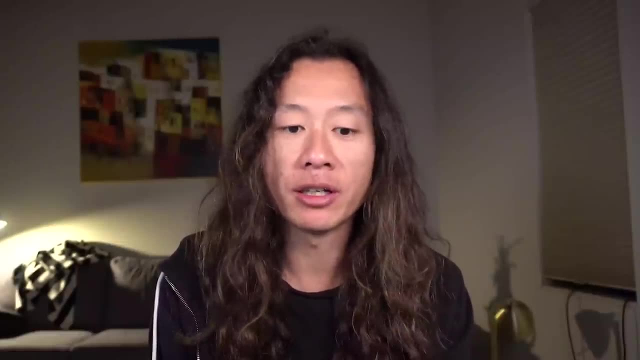 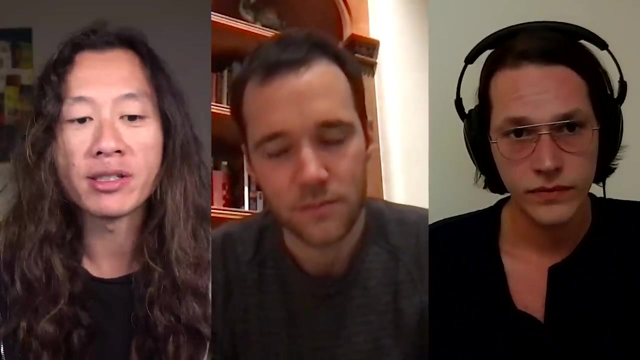 And tell us- like we've talked to some of our partner games, Like people who are launching games, game studios that are building on blockchain, about integrating with Fractal And, you know, tell us about, like, some of the ideas that they've had or ways that Fractal might make an appearance inside of games. 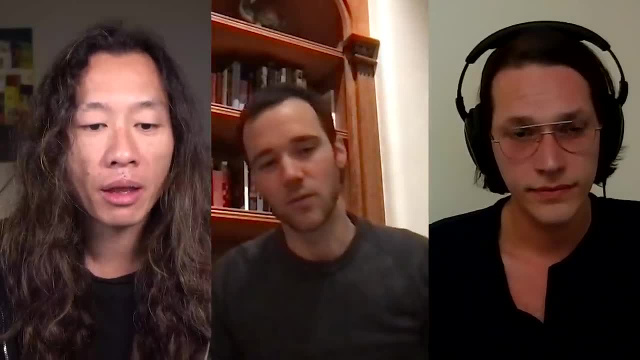 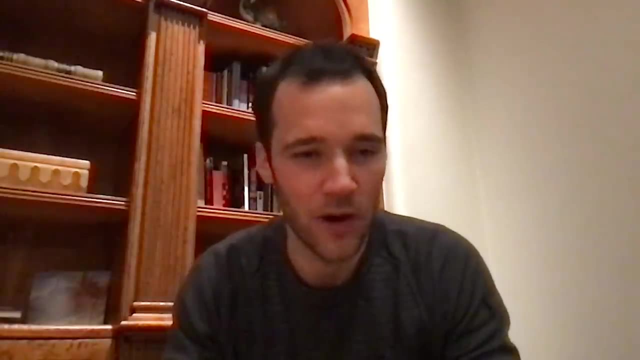 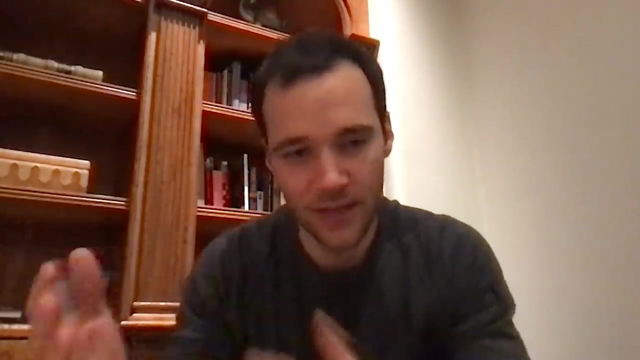 Yeah, I mean- and this is where you know we try not to have opinions right, Because we're – the balance of power and how these games work with respect to you know – the ability to have some skill to up-level versus the ability to pay to up-level. that's a very delicate balance. 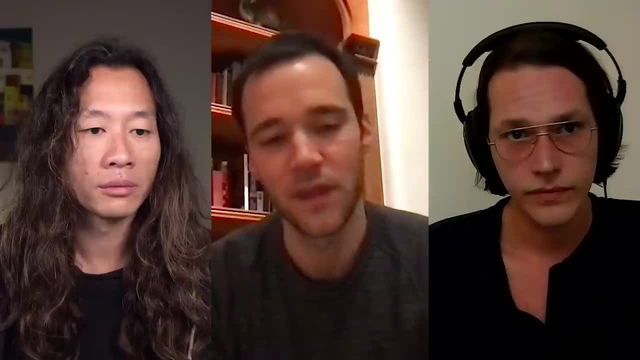 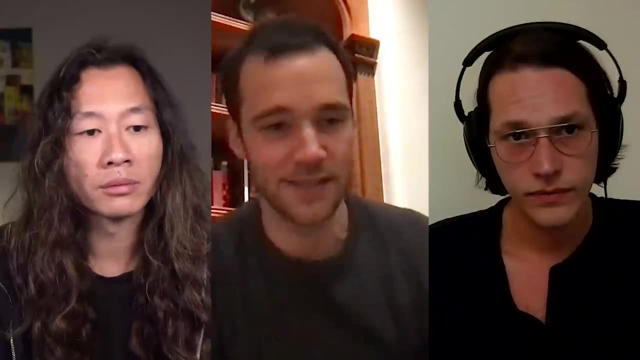 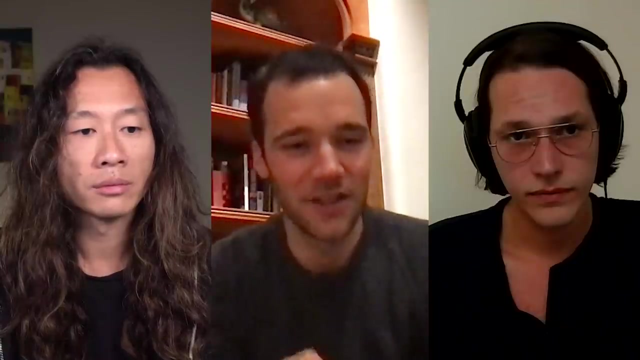 And so these games are all designed very intentionally, And so we don't go into those conversations with much opinion other than the fact that we think that there's this really fantastic engaged community of gamers in the Fractal community that would absolutely love to see the Fractal make an appearance, right. 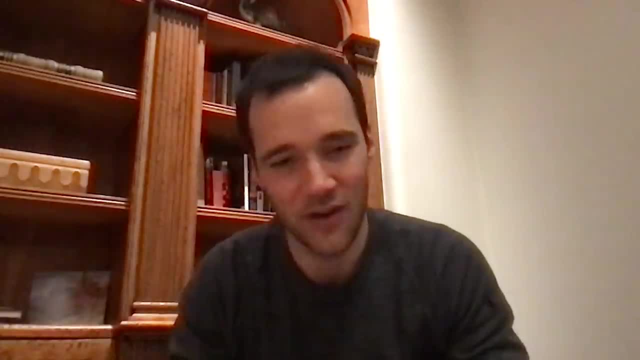 So I think there's sort of like – I think there are two types of integrations that we're going to see. The first is purely cosmetic. You know, maybe Ludovic has a Hexa Fractal And so his tank in Panzer Dogs glows, you know, yellow. 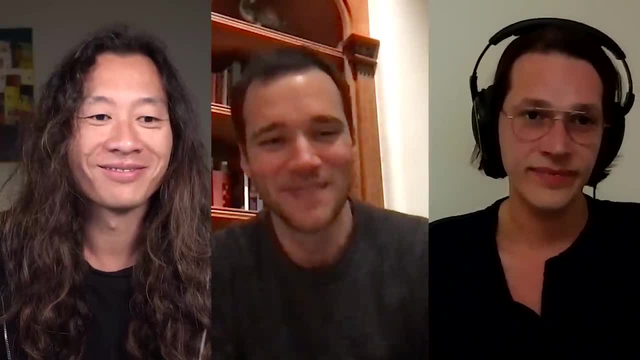 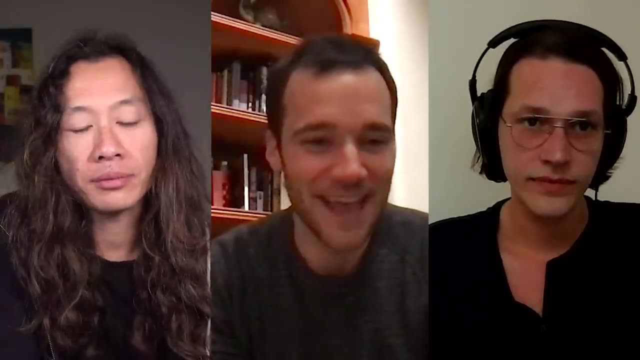 And, by the way, I'm just using that as an arbitrary example not to make any commitments on behalf of Panzer Dogs here, But like everyone who's you know battling Ludovic in his tank – Yeah, It's like holy shit. look at that thing. 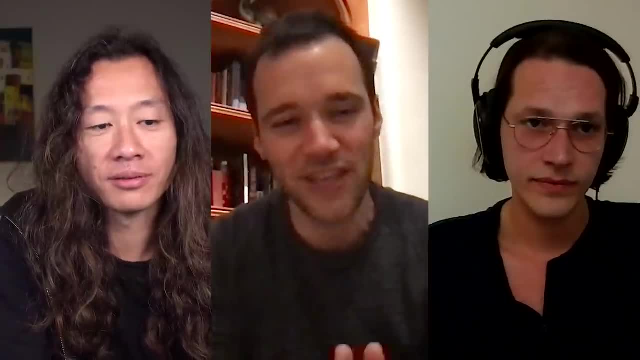 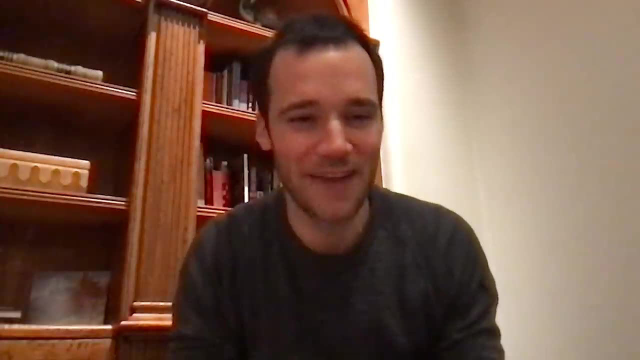 It's like glowing in the dark right And like. that would potentially have no benefit from like in the game and like wouldn't make his weapons more powerful, But it would just be freaking cool And everyone would know that that guy was – you know that guy Ludovic was in the Hexa faction. 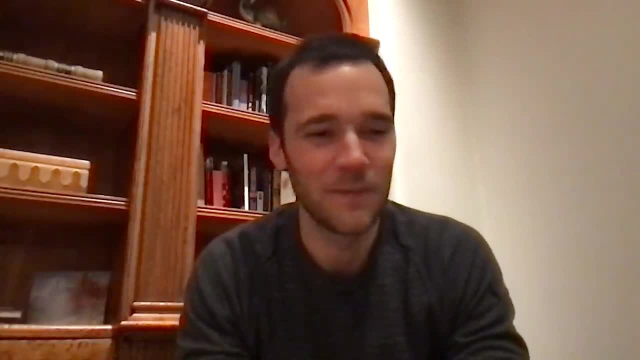 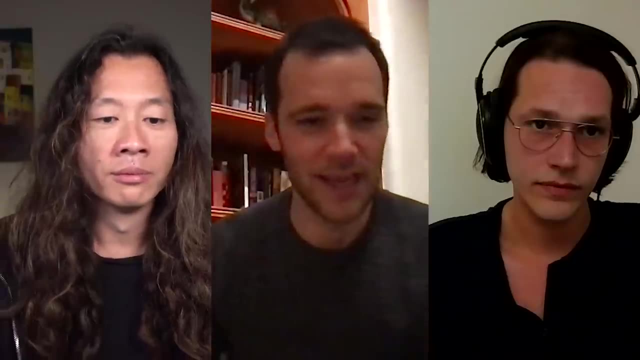 Then there's like – there's other games. I don't want to be too specific, but there's other games that have these like charms and trinkets that you can pick up along your journey, And it's possible that the fractals are related to that somehow. right. 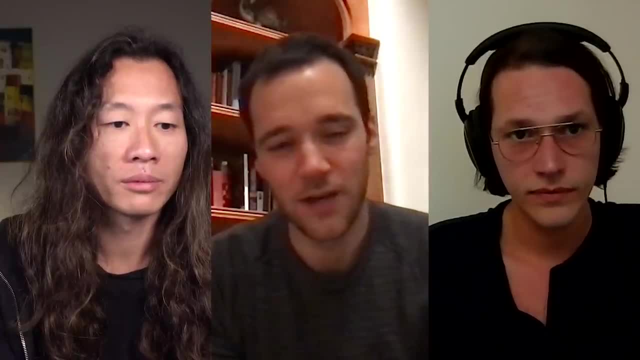 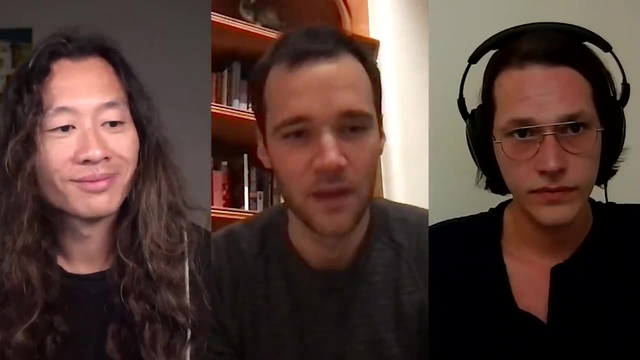 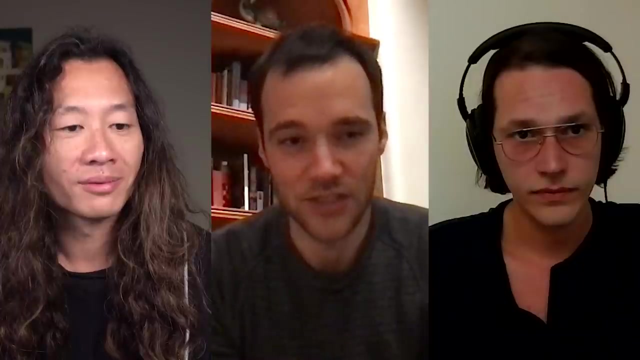 And we're – you know. I'm sure that folks who have spent some time thinking about fractals and maybe have bought some already have seen on our website that we have said from the very beginning that fractals are subject to change slightly over time. 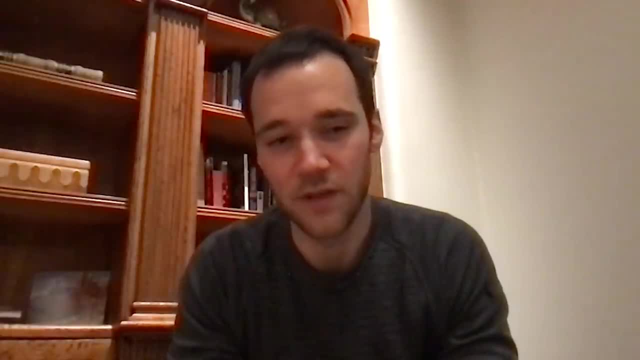 And this is really important to us because we feel like there is so much potential. Like, most NFT collections are static, right, That's what you think of. You think of immutability, the inability for folks to edit, when you think of an NFT. 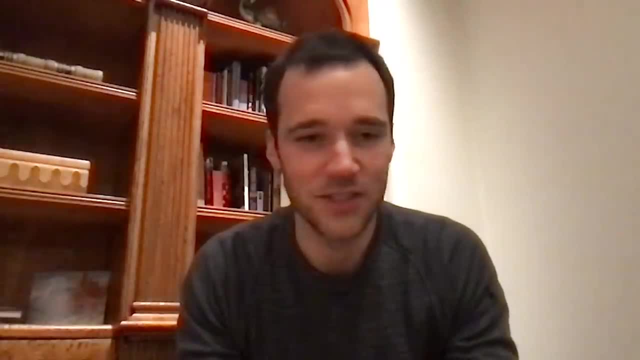 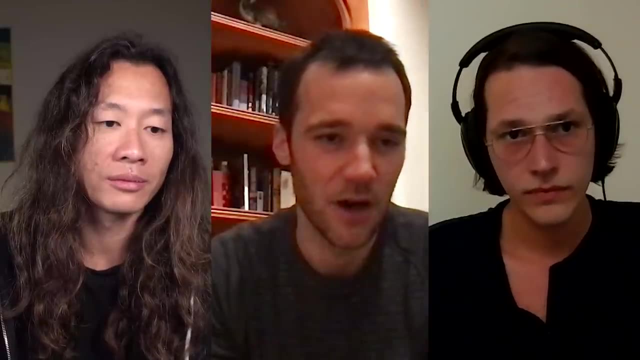 But I think we're at the very early stages of what an NFT means and could be, And I think we've only collectively scratched the surface on like the cool things that they unlock And like I think gaming is going to be one of those. 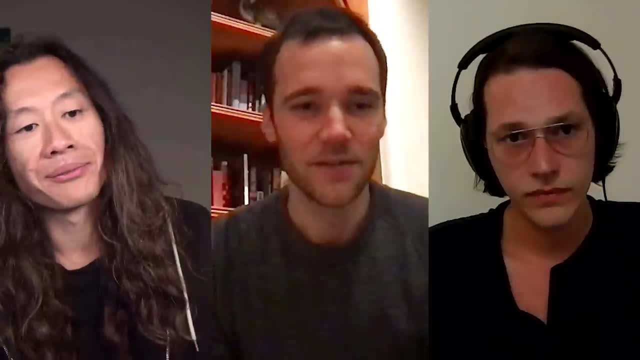 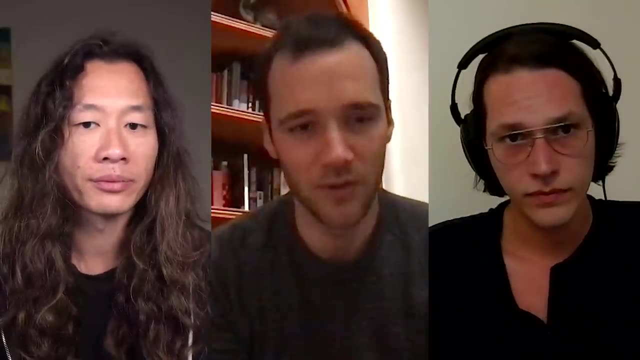 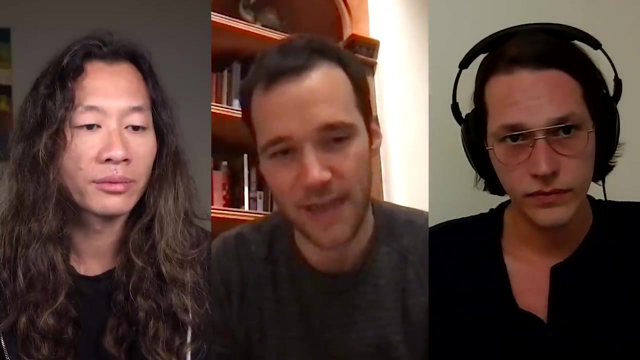 Sandboxes of like, of innovation, where, like, there's going to be all sorts of really fantastic things, But one of the things that is required for some of that innovation is the mutability, the ability for the things to change. So imagine if your power level actually adjusted based on gameplay. 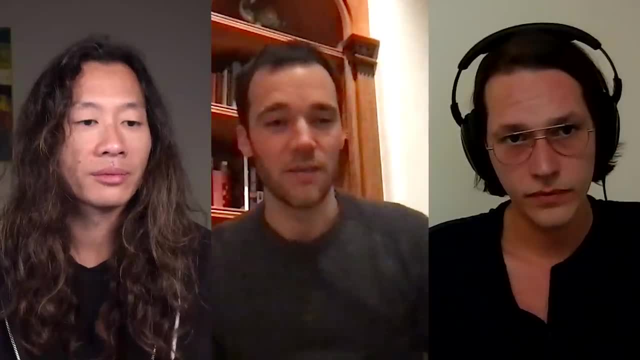 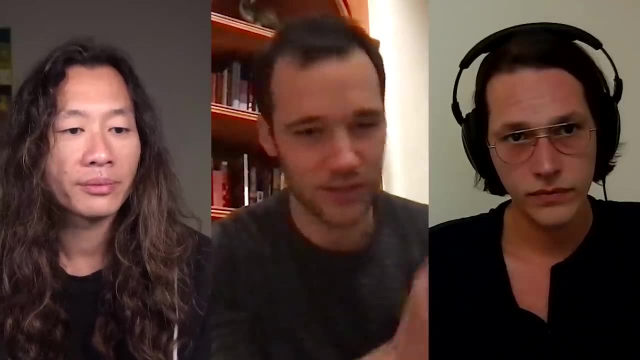 And imagine if, like you could, you know you could go into one game and perform super well, unlock some special benefits, because you're just like such a rock star player, And that in game one, And then actually power up your fractal as a result of that play. 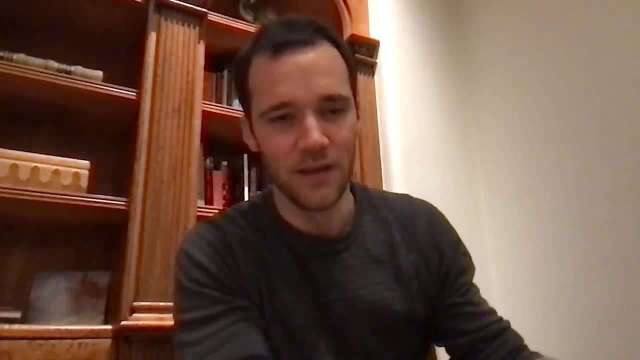 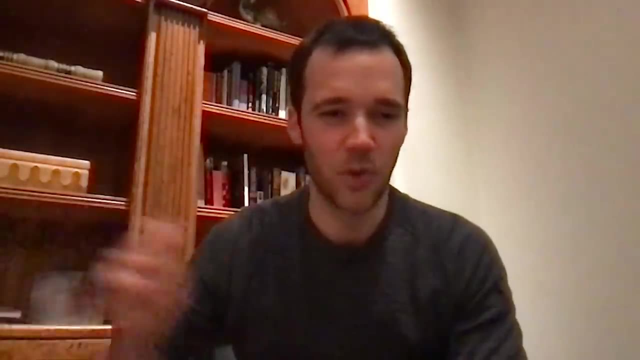 So maybe you actually have to stake your fractal into the game. You know you do your thing, You win your matches, And now you've powered up You could take it to the marketplace and sell it if you like, which it might be worth more than what you paid. 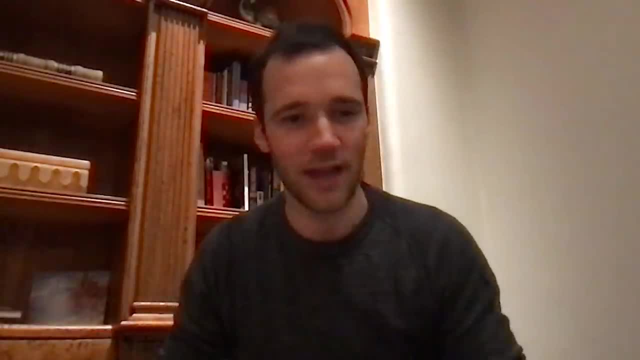 You can go and use it in game number two and now like, unlock a new level because you're at a certain power level. Now do we know for sure whether or not it's going to work? Yeah, Do we know whether this is you know. this vision is going to come to reality. 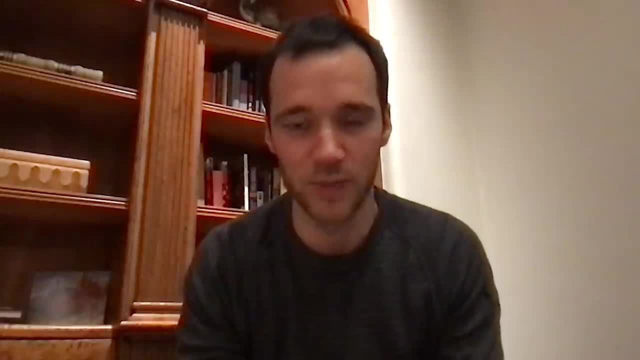 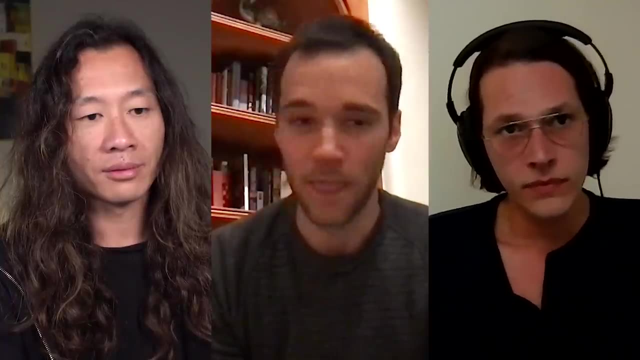 No, I don't think so, But we definitely think that there is a huge potential for these types of interactions across game And we wanted to be the- you know a company that actually helped bring that future forward, because it's a really powerful vision.